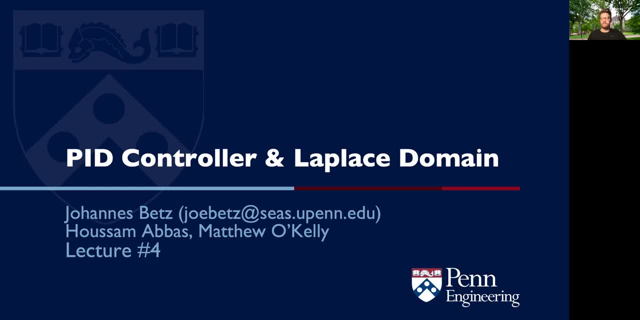 of our vehicle and the Laplace domain will give us the possibility to analyze the PID controller in different parts of our vehicle, and the Laplace domain will give us the possibility to analyze our controller or our control system later. So what we will do in this lecture is, first of, 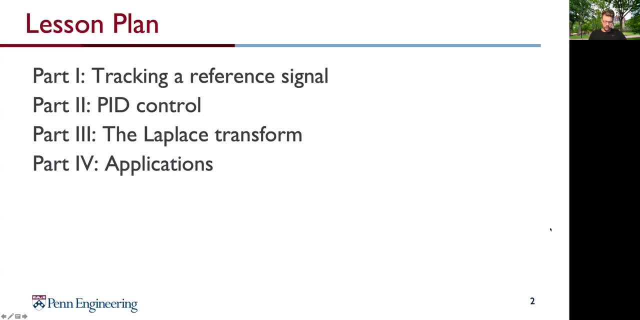 all that. we show you in an introduction. the tracking of a reference signal. What does it mean to have a reference signal and what does it mean to track such a signal? On the second part, we will make a deep dive in the PID controller. We will show you on the 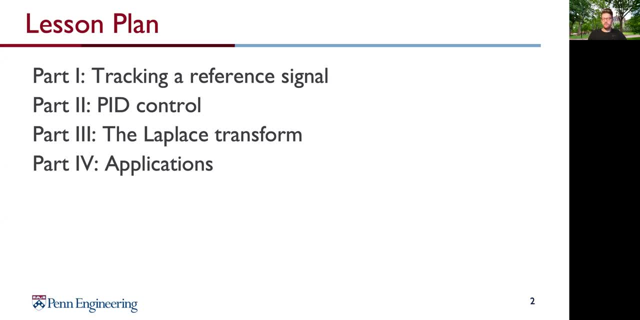 example of a path tracker. how to apply a PID controller. Part number three will be the analysis of a control system with the Laplace transform. Here it gets a little bit more mathematical, but no worries about that. And number four: we will show you a first application where you can find 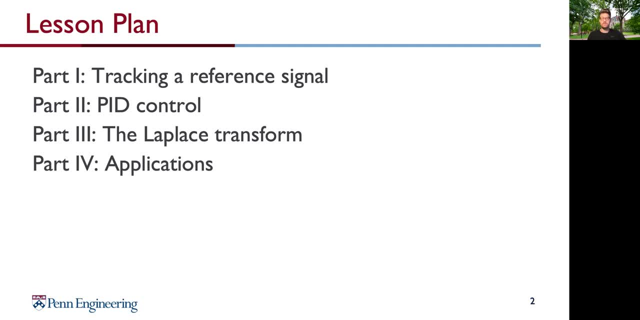 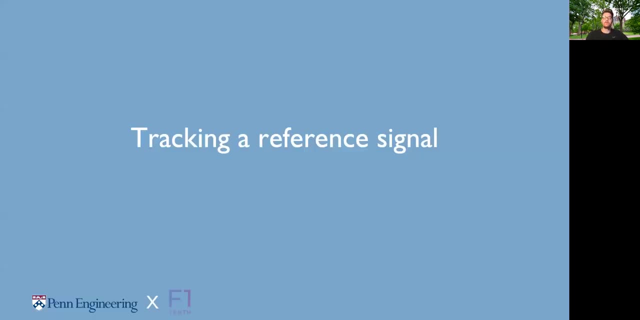 all the knowledge from part two, the PID control, and part three of the Laplace transform. My name is Johannes Betz and today I will show you all of these topics. Let's start with number one: tracking a reference signal. So, first of all, what I 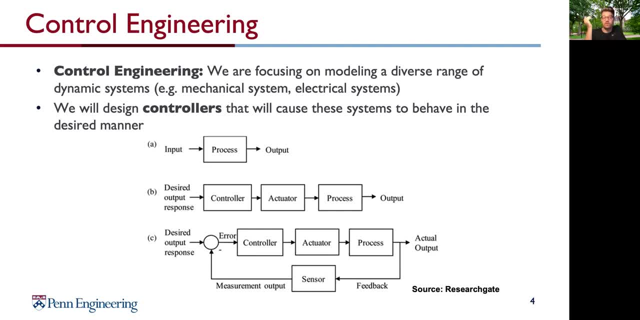 will show you today is like what is like controlled engineering. I think you- all of you- heard that in your engineering courses before and in control engineering, we are focusing on modeling a diverse range of dynamic systems. We can think about mechanical systems, we can think about electrical systems, and for all of these dynamic systems that have 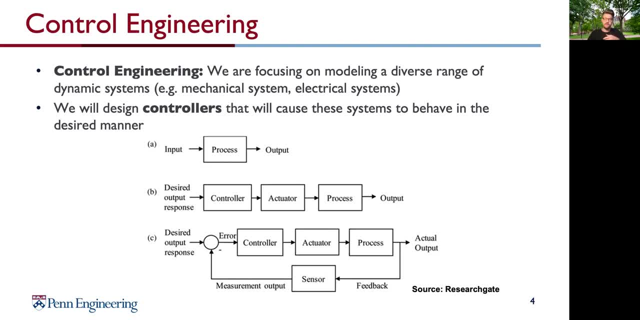 moving parts. this has like electrical currents have flown. for example, we will design controllers that will cause the system to behave as a desired manner, which means we want to do the system something like our car, to stick to one path, to design a controller that is applying specific parameters to our system. here. 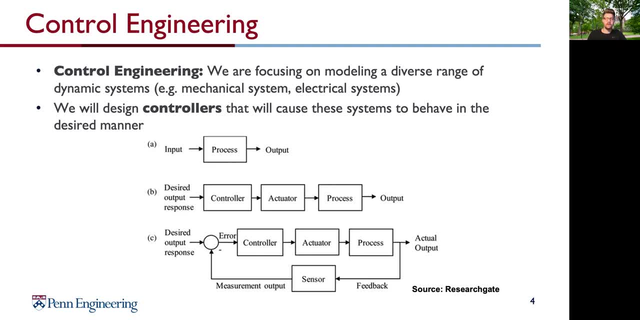 is for you to remember what are the different types of modeling you can achieve. it's like you have a simple input and output with a process like for sing something with them in B. you see here that you have feed forward controller, which means that you have a desired output response that you want. 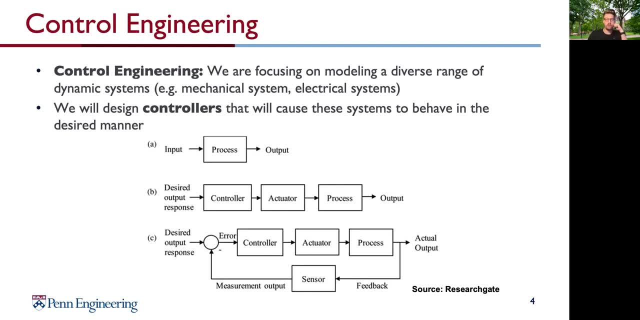 your system to achieve something, UN apply a controller and you have an actuator that achieve something later and you have an output that is this simple. then the process of design, the system in B, can be integrated into a follow-up application. so I've just presented this for you as a general. 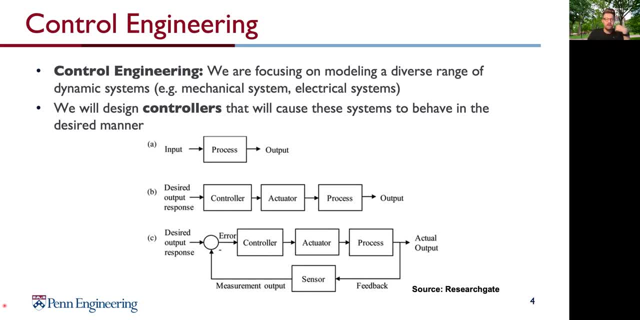 that is your desired output, as before. and in the last part, this is the most important part for all, for us today. therefore, I wish highlight this. this part is what we want to achieve. we have a desired output response, we have a controller, we have an actuator in a process and we have an actual output. 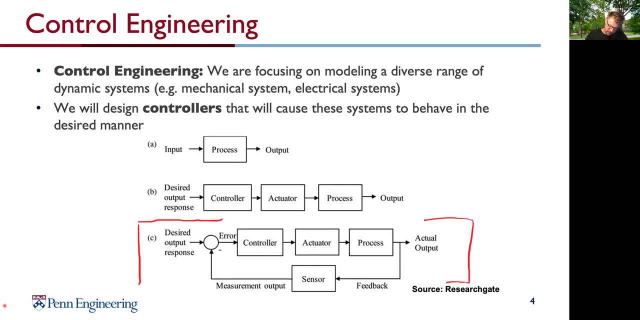 afterwards. but this output is better than in this output here because we are having a feedback loop and in this feedback loop we are integrating a sensor, we are integrating a measurement input that is creating an error afterwards here, and this is what we do in control engineering. we design such 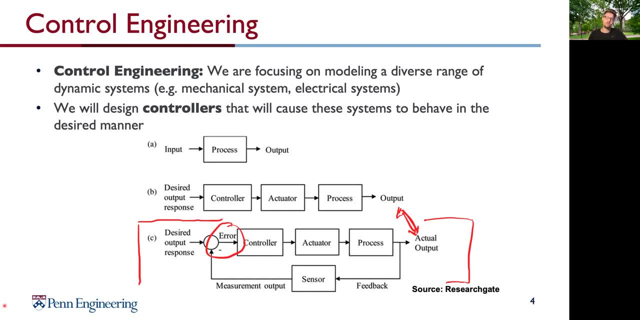 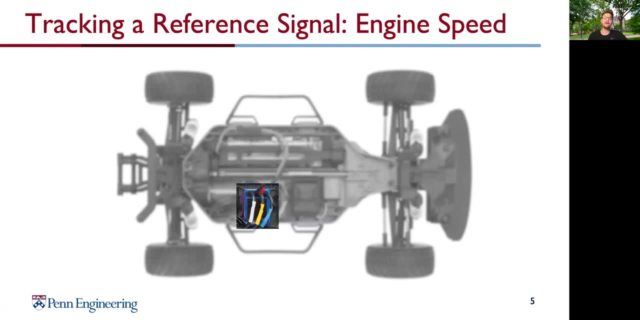 feedback you the loops in the controller to achieve the desired output afterwards. so, for example, imagine we have our f1 tenth car here. what you can see here the highlight is the motor controller of the car. what we do? we want to track a reference signal to achieve a specific engine speed. so what we do, we hand in our 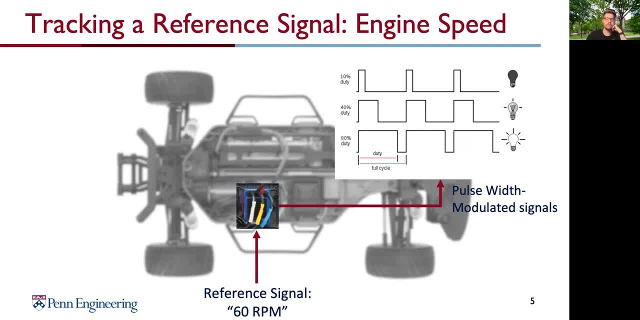 reference signal- in this case it's 60 rpm- to our controller. the controller is generating a signal. in this case it's a pulse with modulated signal. this pulse with modulated signal has always a specific duty cycle, a full cycle. what you can see here, this full cycle has one part which is a digital. 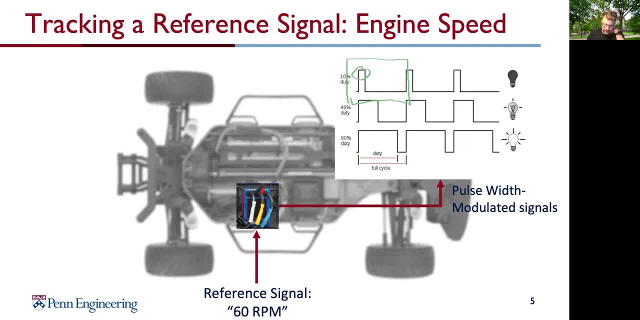 one- what you can see here- and his one part, that said, which has a digital zero- what you can see here- and by shifting the lengths of both parts we can achieve a PV, a so-called PWM signal pulse with modulated signal. this pulse with modulated signal, then, is going directly into our motor, our electrical motor, and 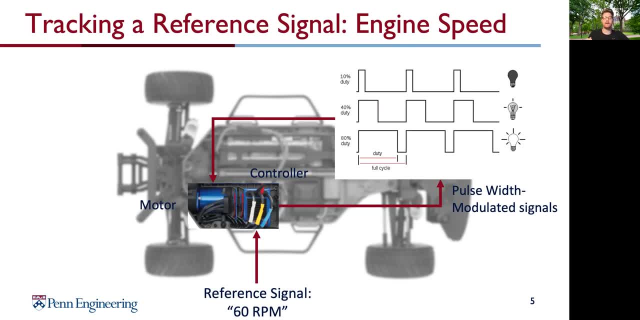 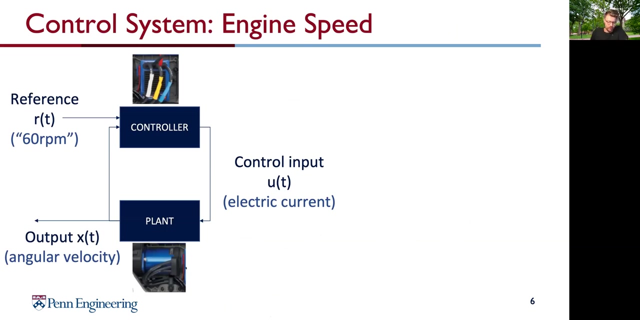 this motor is achieving an electrical current with this pulse, with modulated signal, and is outputting a motor speed or an angular velocity. but this is our physical system here. if we are in the field of control systems and control engineering, we will describe it a little bit more different with our control system. here again we have our 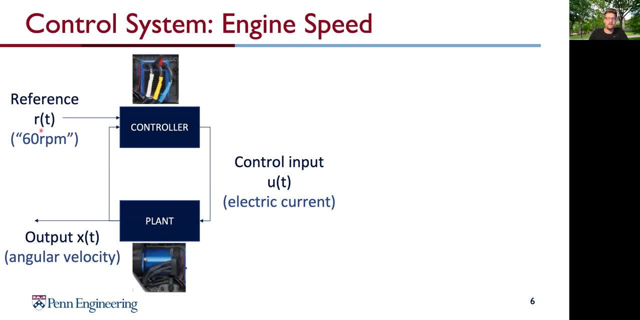 reference signal, which we call RT, with 60 rpm here this signal is going inside our controller. the controller is generating a control output which we call u from T- here in this case it's the electrical current- and this information is going into our model plant, which is 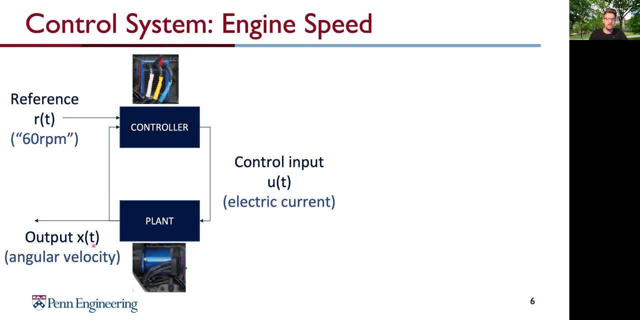 the electrical current and this information is going into our model plant, which is the motor and is creating an output X from T here. we will see here now the signal where you have the control input, which is our electric current, in blue, just like a zigzag here, and we have followed afterwards in green here the 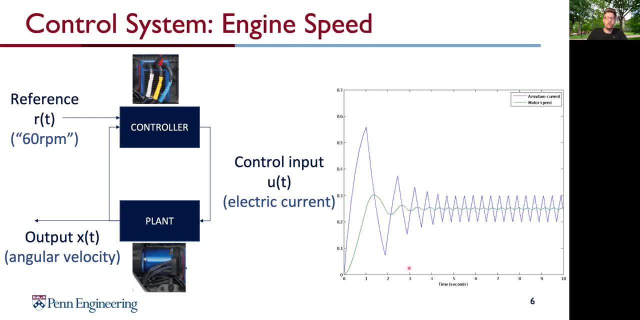 response from our motor who is trying to achieve a desired speed. it's going a little bit up and then here is achieving the speed afterwards. this is what we mean when we say we want to track a reference signal. here it's 60 rpm. how we can do that? we have to get to a higher control input or higher electrical. 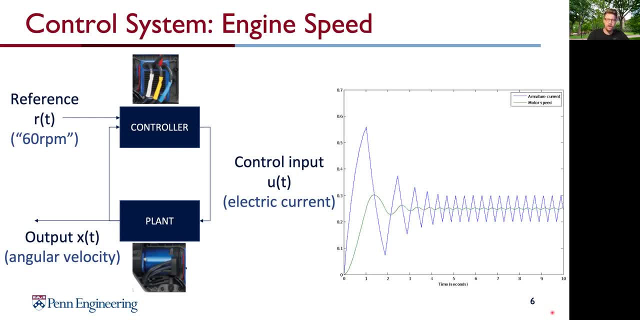 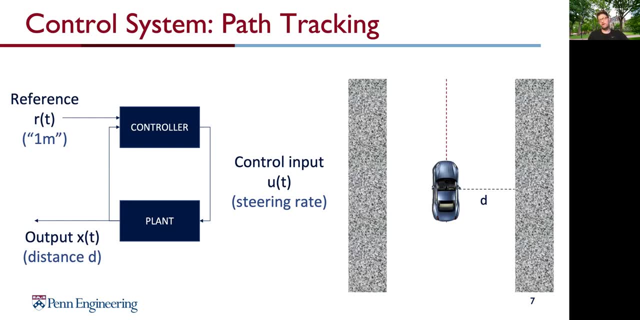 current and afterwards we receive the signal and the same. you can imagine what happens when you have a high electrical current and you have a high voltage current, when we're thinking about autonomous driving. in autonomous driving, we want our car to stick to a specific path, a specific way. 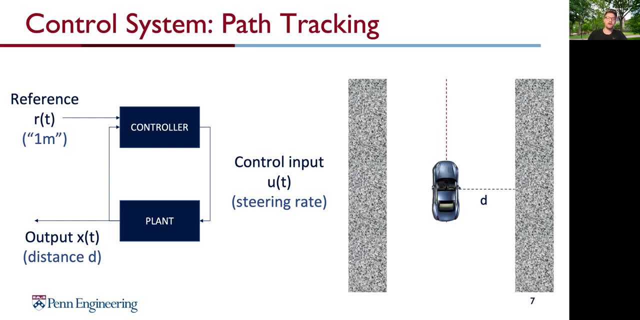 we define in advance and we want our car to stick to this path, and what we are designing here is a control system. in this case, the control system has an reference signal, R from T, which is like one meter. we designing a controller, and this controller is calculated. 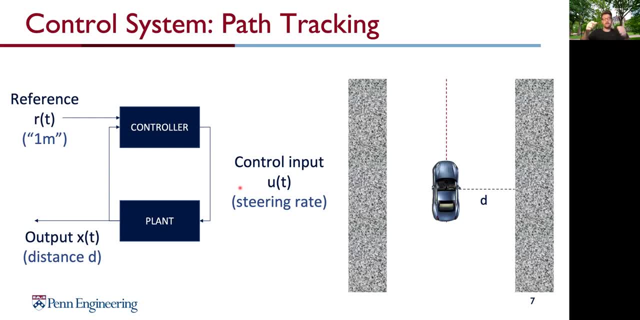 again the control input, which is here the steering rate of our car. this is the same what we people, we humans, are doing with a car: we applying a control input and we decreasing our distance D, for example, to the wall, which is afterwards the output for our system. but this is like an open-loop system. we want to be a. 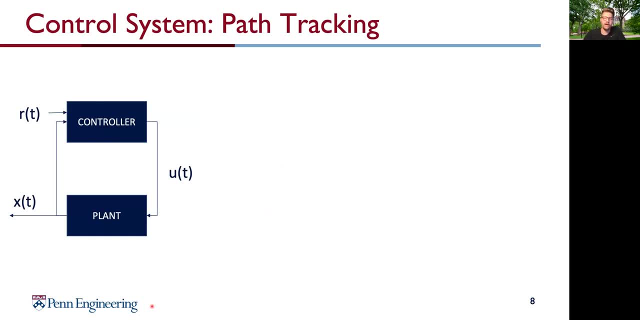 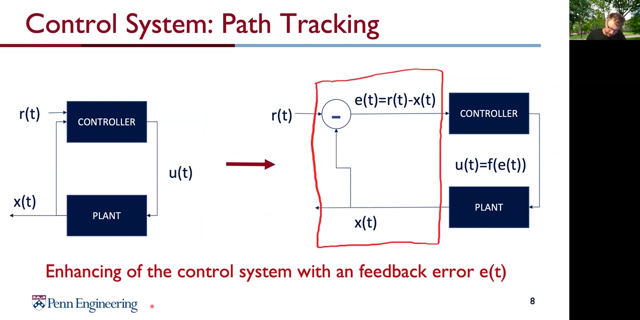 little bit better because we want to enhance our control system with a so called feedback error. this feedback error, what you can see here- is generated by setting up a loop where we feed feedback, our output signal, here back to the reference signal and we calculate it with. we have our reference reference signal from T. 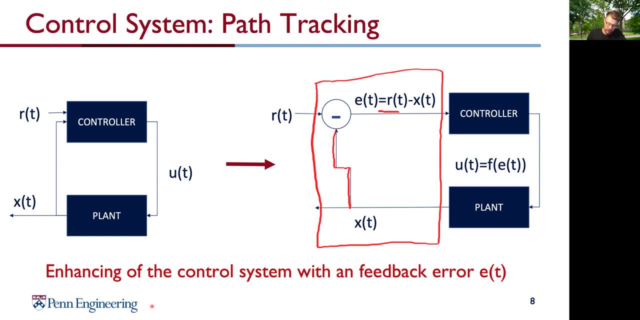 and minus our feedback signal X from T, and this is how we can achieve an error, and therefore we are not only inputting our reference signal anymore, we are inputting the difference between our decide reference signal and the ejercised signal, which is our signal. and what we are doing here is we are 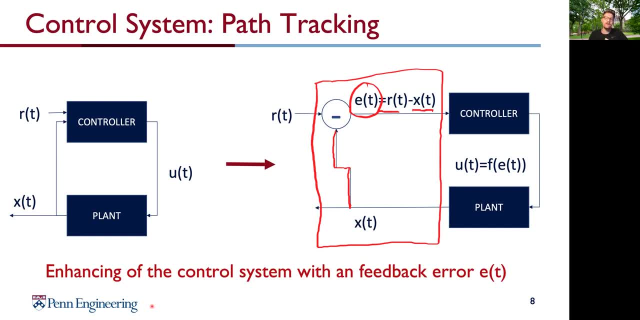 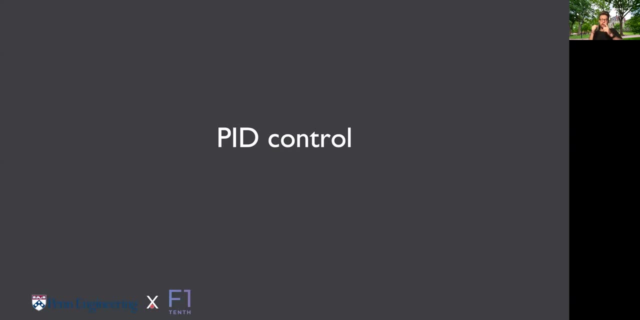 actual output signal, which means we are getting here much closer and much faster to our desired system output, and this is what you need to know when we talk about tracking a reference signal. you have to remember how to set up your control system, which means you have to define for yourself what is the reference. 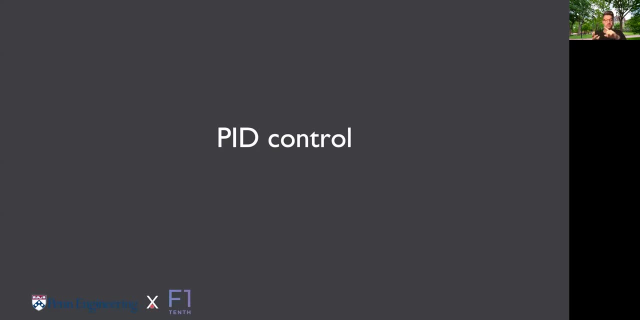 signal? what is the control output signal? what is the control input signal? you have to define for yourself. where is the feedback loop? so which information do you need to feed back into your system? we will learn later with the car that we have to measure the information, additional information to create a much. 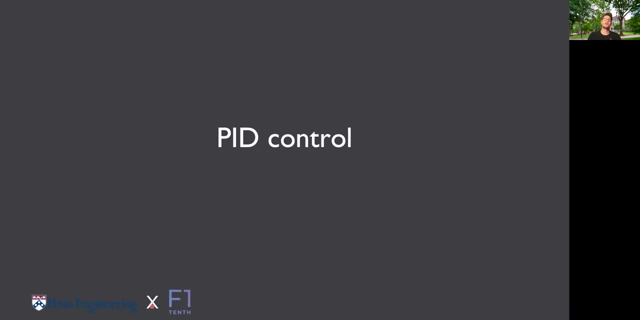 better arrow, tracking arrow or let's say, control arrow for our system. this is what you have to remember from part number one and part two and part three and part four and part five and part six and part one. now let's step back or let's step forward to part number two, the so called 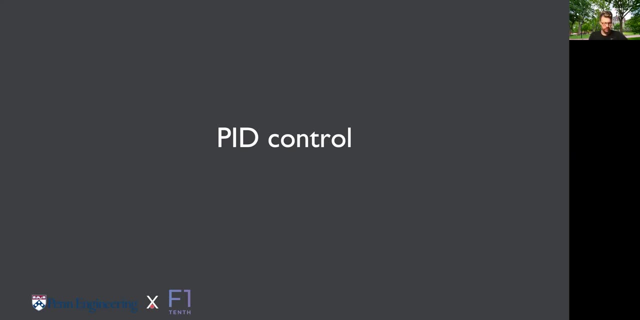 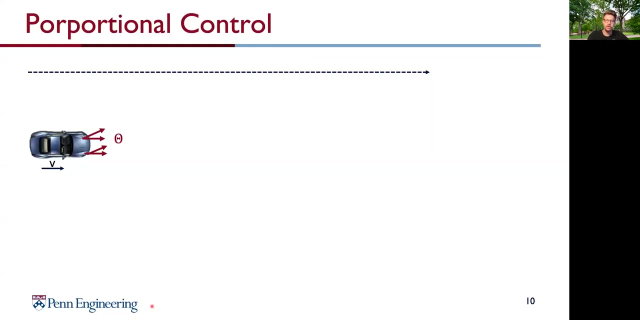 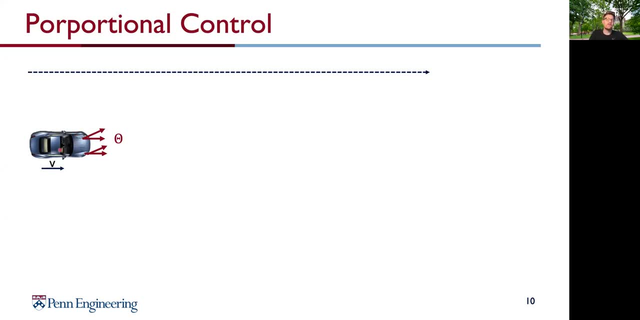 and you. this car is driving with velocity here. this is a constant velocity and you, as a normal car, you can choose the steering angle, which means you can steer the car to the left or steer the car to the right, and the goal is that this car is following this line. here and now there's a question for you. 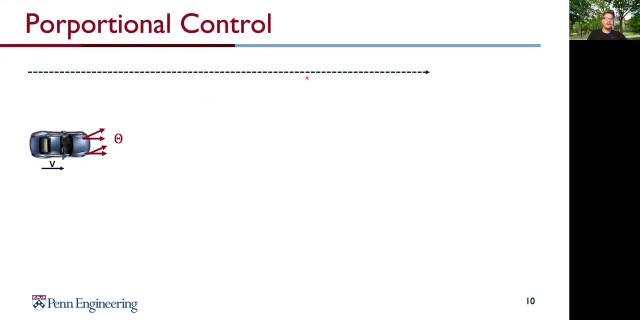 how can you achieve to follow this line here? do you set a random steering angle? do you set like a constant steering angle for our car? so what do you think is the best way to achieve driving at this line here? okay, obviously, a random steering might not be. 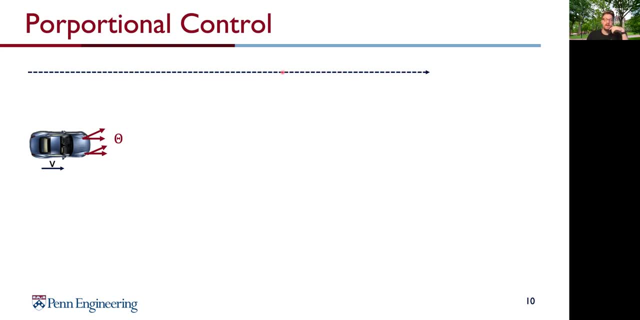 helpful here and an additional constant steering would lead to a shoot over here. so what we can do in this special case? we set up a special variable for us. in this variable we call the cross-track error. this cross-track error is measuring the distance from the center center mass of gravity of our car to our 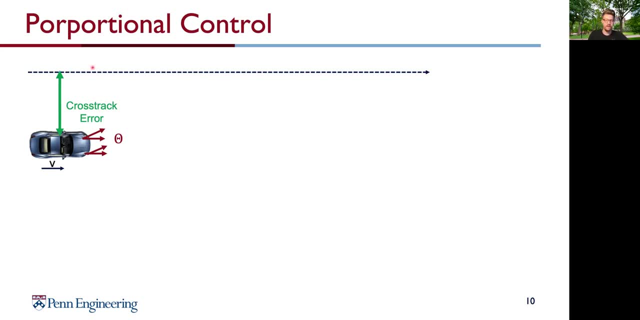 reference line or the line we want to drive it, and what we say now, we, or the steering of the car, must be in a proportion to the cross-track error, which means we have a so-called proportional, or the abbreviation P, controller, and this is the complete magic we have here. so the idea is the 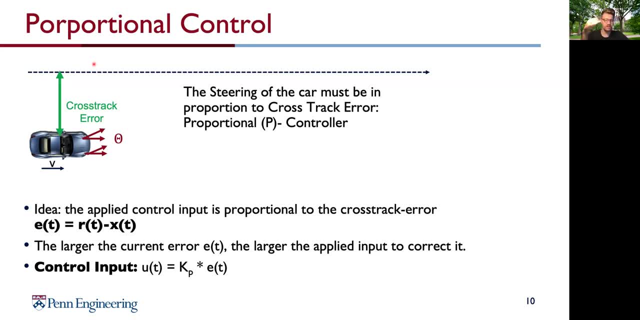 applied control input is proportional to the cross-track error. so we have it here again. our error is the reference signal minus the output signal. the larger the current error E from T is, the larger is the applied input to correct it. which means if we have like a high cross-track, we have a high steering. 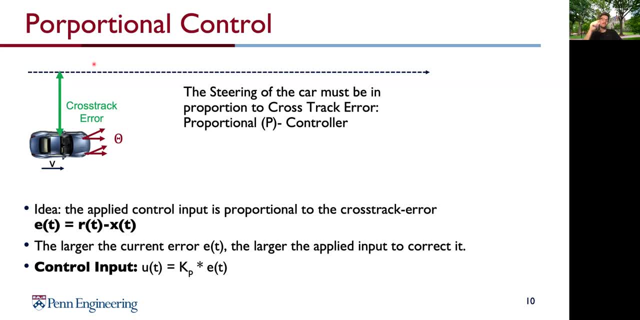 angle. if we have a small cross-track error, we have just a small steering angle and the control input we generate you from t is that we multiply our cross-track error with corresponding�� gain, a gain variable, K, P, and this is the magic behind the proportional control. 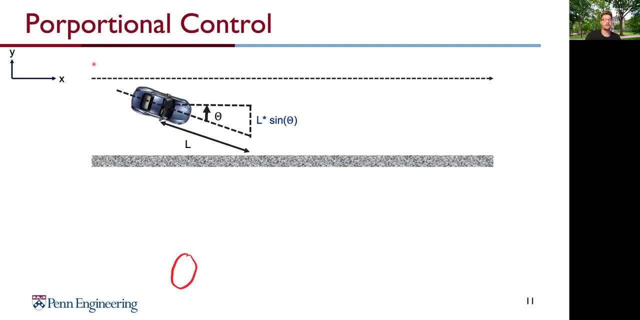 but we will now go a little bit more into detail there. I enhanced our setup. I give you here the coordinate frame X and Y, and we are driving here again with our car. and what we are saying now. first of all, we want to drive on the reference. 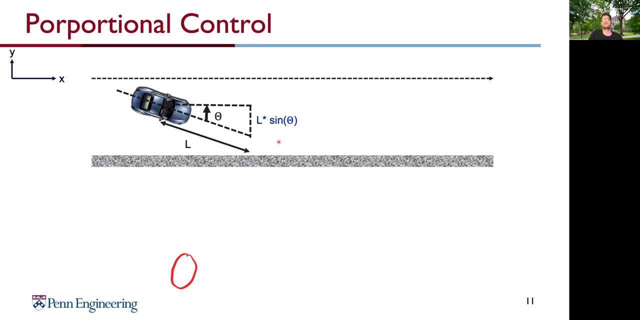 line here and we want to drive parallel to the wall. so again we have our control input, which is the steering angle, and this is the output we. this, the control input, is our steering angle and this is where we achieve the final movement of the car. again, the velocity will be constant here and the goal is keep the 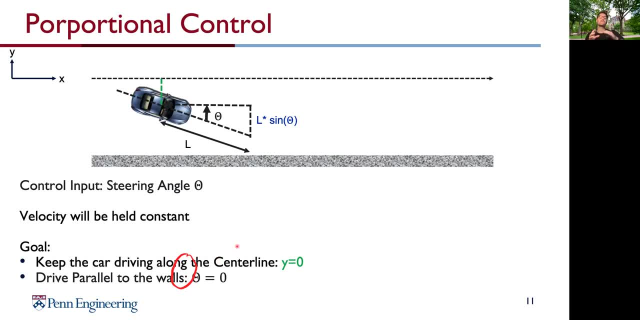 car driving along the center line and the steering angle will be constant here. and the goal is keep the car driving along the center line, which means from a mathematical point of view y must be zero. and then we say we drive parallel to the walls, which means our steering angle, theta, has to be. 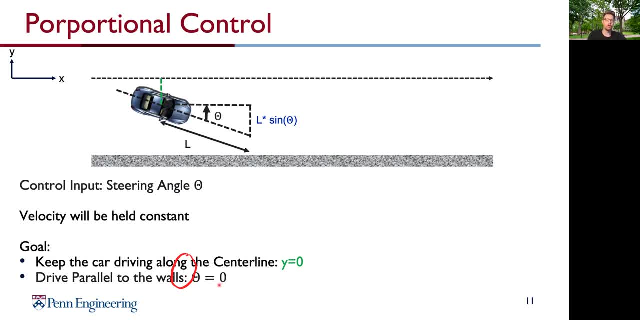 zero. but this here is wrong. we need, like, a better way of displaying that we are driving parallel to the wall, which means that are cannot be achieved to be zero. what we do better is that we say we multiply l by the sinus of theta and want this here to be. 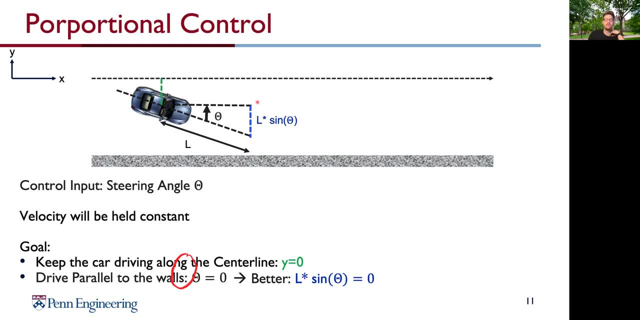 zero, which means the distance we calculate here from the car needs to be zero, which means the better way is, after driving l meters we want to be still on the center line, so we will minimize the horizontal distance after driving l meters and this gives our car a little bit more time. 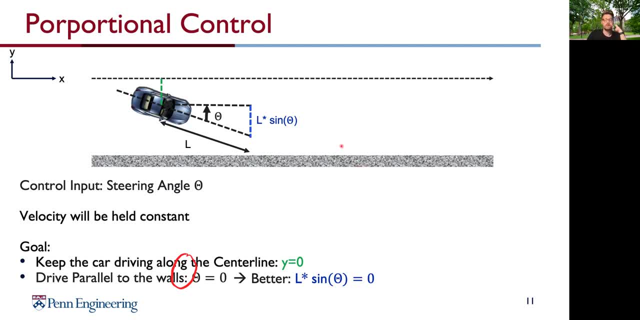 to achieve the center line and not focusing on theta zero only here. so again, our goal is to keep the car driving along the center line. why is the distance from center line and l multiplied by sigma? theta is the difference between the distance between the center line and the center line. 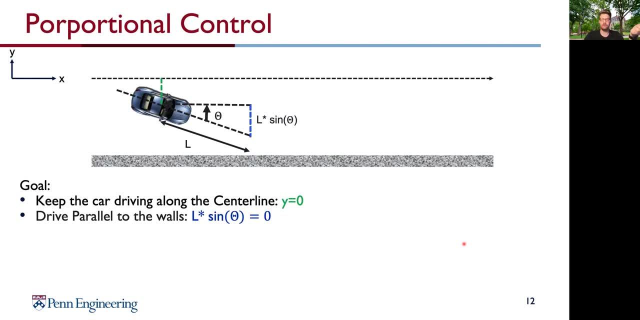 now, this is a very fewходer relation and it also will repeat itself to say, for example, the distance between the center line and the center line is zero. right, i will devoir dreaming about m? i-theta 양-instrument. and now our crucial percent is the distance between the center. 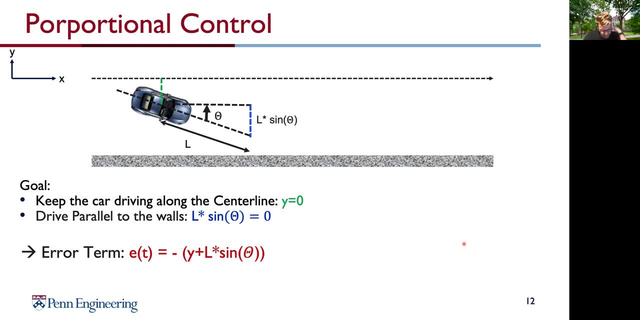 line and the center line, the distance between the center line and the center line. this includes especially the distance between this instrument on thisவ 있어 daqui BE Artemia and Alexandra and 안 as, and this is our error term here. so now we achieved to set up a mathematical function that defines our 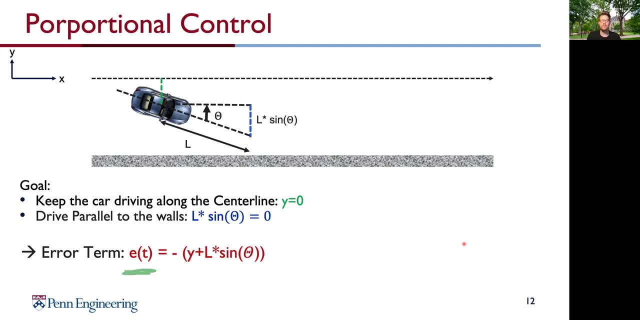 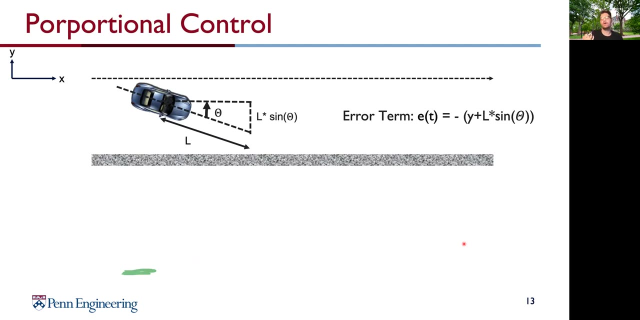 error term and we want to minimize this error term. this is our overall goal. so now we have defined the error term on a medical mathematical expression and we can check now if this is valid for us. so first of all, we can check if Y is bigger than zero, which means our car is on the left side. 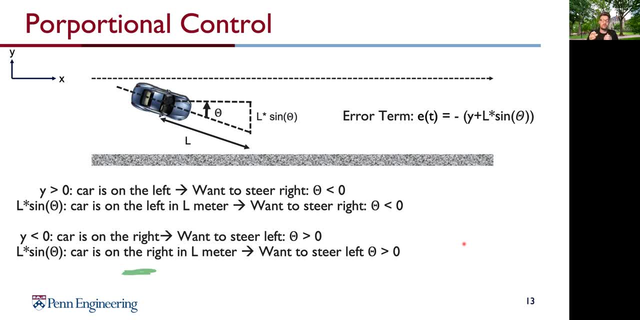 which means we want to steer to the right, which means afterwards that R needs to be less than zero, and again L multiplicates the error term and we can check if we are good for us. so now we can by sine of theta, which means the car is now on the left in L meters, which means 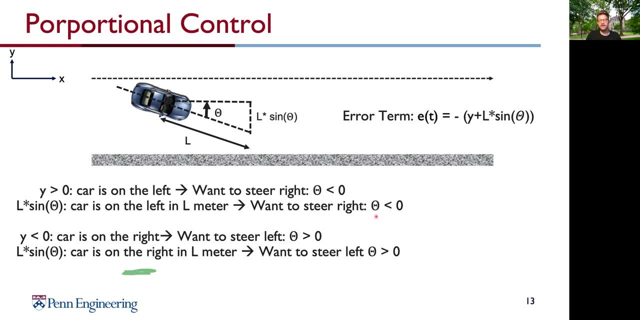 we want also steer to the right. theta is less than zero and complementary here. if Y is bigger than zero, the cars on the right and L multiplied by theta, the cars on the right in L meters and also both set us, are bigger than zero, which means our calculation. 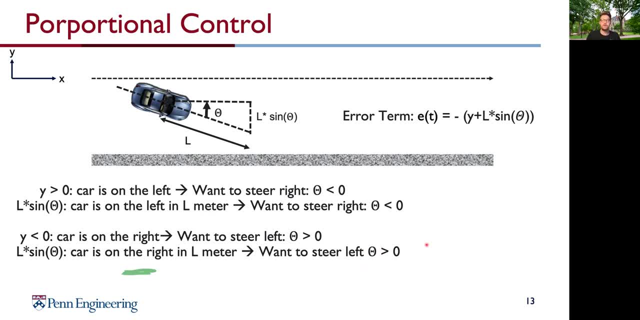 is correct here. so what is the overall conclusion for us? our metamagatam, etical expression: we have to set the desired angle. remember here, we have our arrow here and we set about the same angle. we have our arrow here and we set about proportional control, which means the desired angle. theta D is our sort of 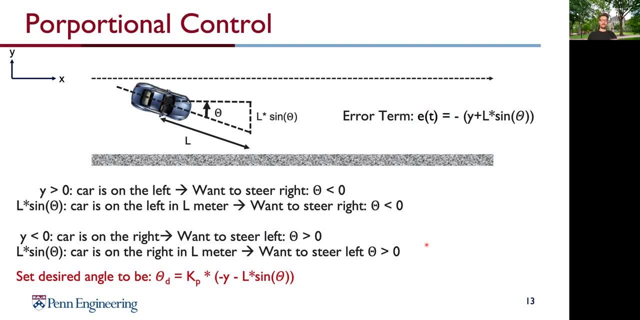 that is our KP gain multiplied by the arrow, which means minus y, minus L, multiplied Senos theta, and this here is now our mathematical expression. with all the available physical parameters we have, we can easily calculate to create our proportional control. now here is a small video for you where you can see. 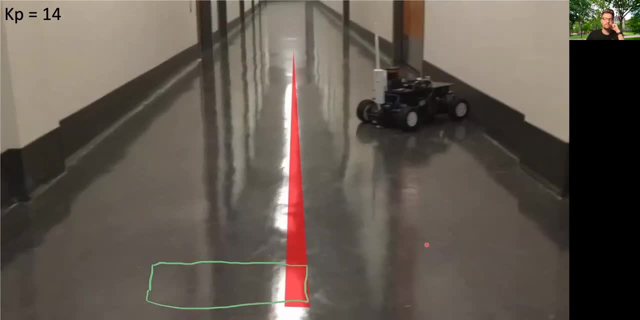 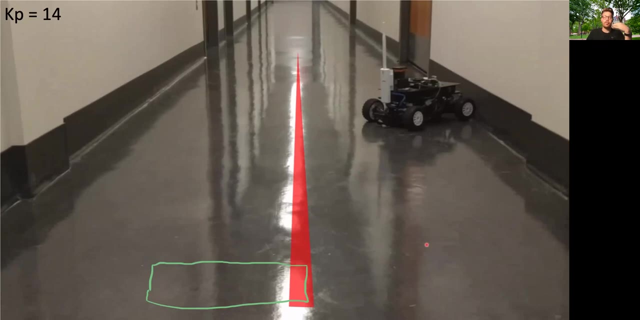 where we set up such proportional control. what we see here we will overshoot with this algorithm. algorithm very easy. the car will oscillate around and this will oscillate around this um center line, or the um, the center line we try to follow really easy in that way, which means we need to tune this parameter first of all so it works out better. 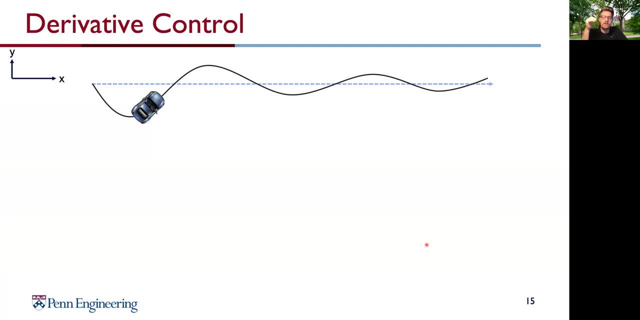 so what is good about the p controller, the controllers or? the p controller improves the steady state accuracy by decreasing the steady state error. remember, the steady state error is defined as the difference between the input and the output of a system in the limit as time goes to infinity. in addition, the p controller, as the steady state accuracy, improves the stability of 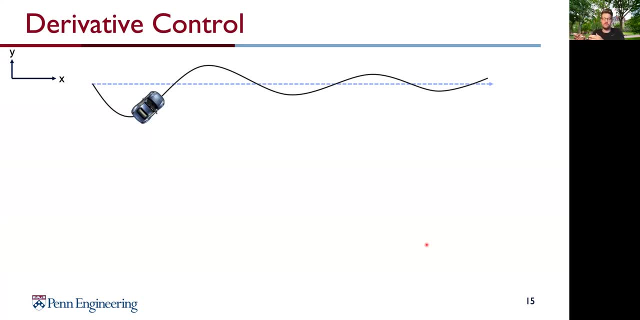 our system also improves, and what we always want to achieve in the control system- that it is stable. in addition, the controller also helps in reducing the unwanted offsets produced by the system. what's bad in a p controller is due to the presence of a p controller, we got some offsets. 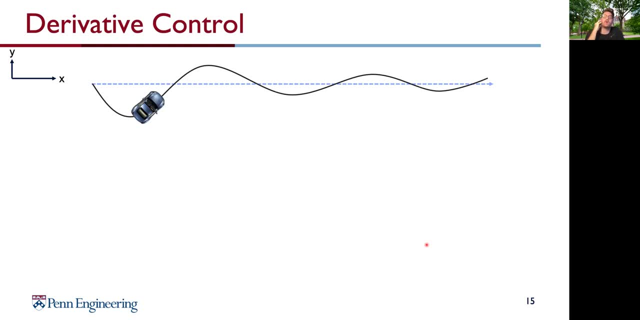 in our systems, and the proportional controller also increases the maximum of the overshooting of the system- what you can see here- which is achieved by a p controller. so what we have to do is to modify the p controller. so how we do it? first of all, we can do this by returning a 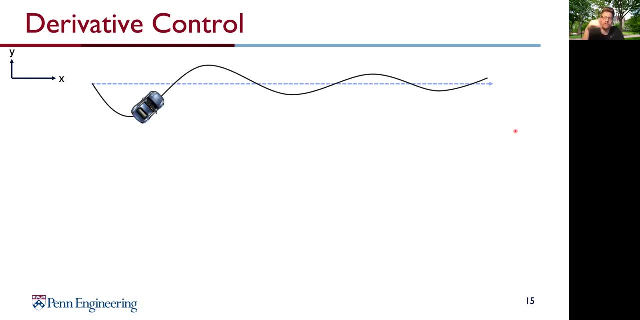 p controller and by using our p controller- let's say a p controller is doing a bit of work- we can add a p controller to our p controller, so we can modify the p controller. what we need to do is to add an a p controller of this b controller to our c controller and we can emphasize the. 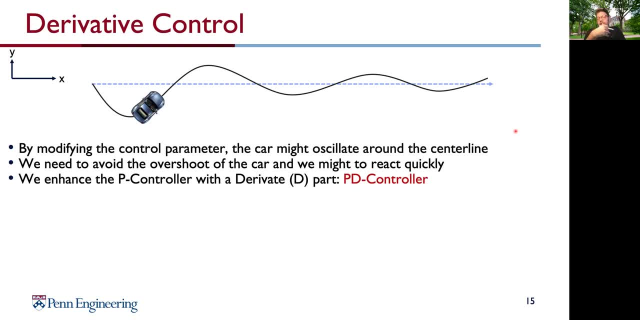 control command and to increase the speed of the p controller as the p controller gets more and more fast and faster as theanteer is active. so now we are getting a little bit more advanced. so how can we advance our calculation so it's receiving better results? so what we need when the car is turned, enough to reduce our defined error, it won't just not overshoot the centerline only. 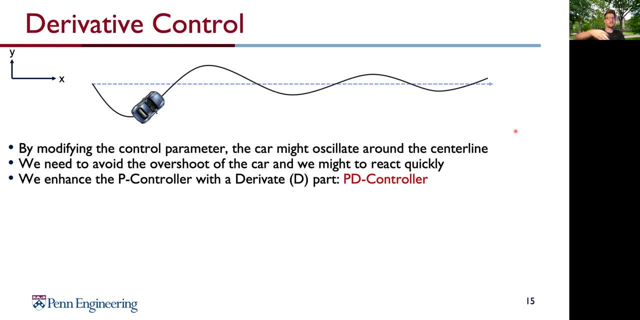 so we need our card to react a little bit more quickly, because the peak controllers, yeah, also really slow because the car needs time. and we can achieve that: that we integrating a second part, the so called derivative part, the D part, and therefore we create a PD controller. you can imagine like this: we will now 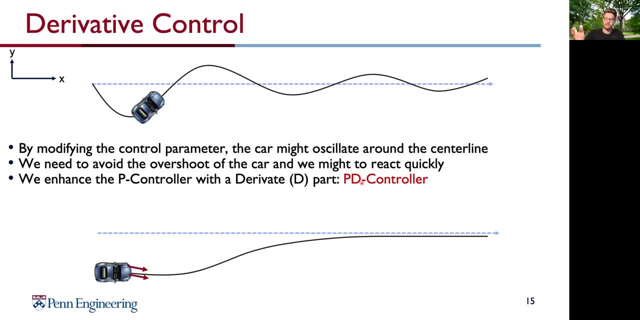 approach the centerline more slowly, but steady as we approaching this, steady as we reducing the error. so when a car is turned enough to reduce our defined error, we integrate the new term. so our car figures it out that it can steer like to the other side again because it's. 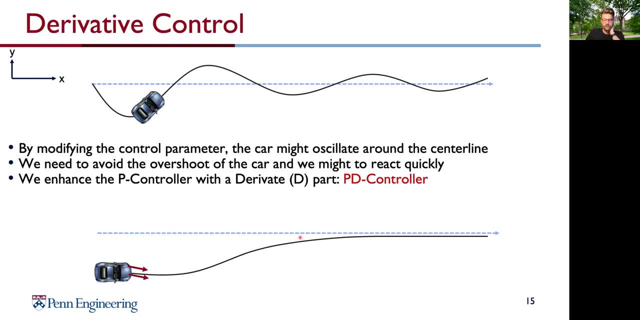 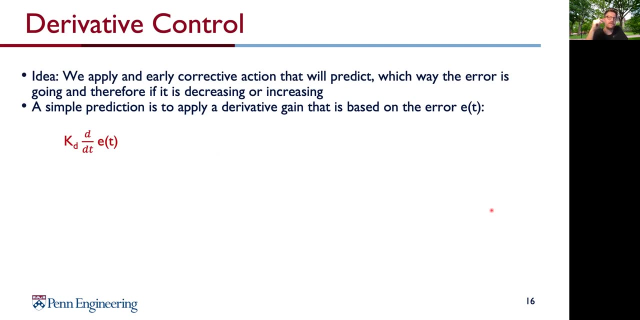 approaching the arrow itself, the car will count the steer, or like steer up, and we approaching this curve, this curve, more smoothly. so the idea is now: we apply an early corrective action that will predict which way the arrow is going and therefore, if it is decreasing or increasing. decreasing or 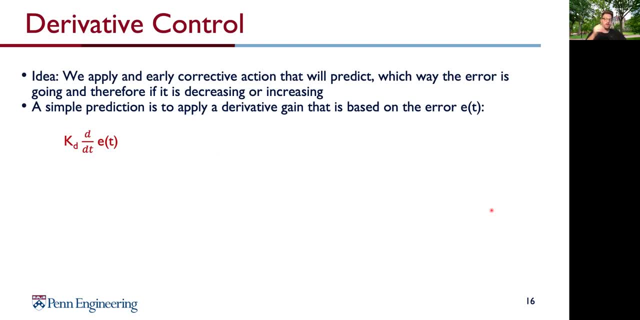 increasing. this is our word for a derivative, which means a simple prediction is to apply with a derivative gain, and this is also based on the arrow. so now we have our new derivative gain, KD, and we have our derivative part, which means the ET do DT. so we add this. 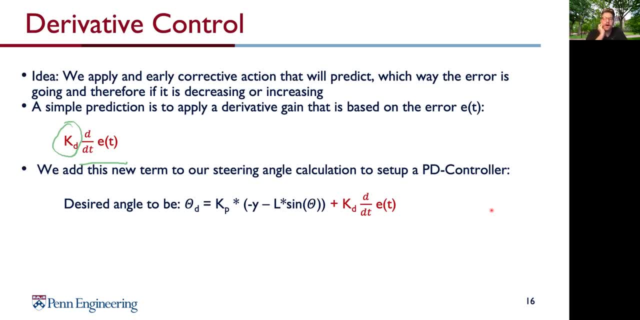 new term to our steering angle calculation for our PD controller setup, which means we now advance our P controller to the D controller and have now integrated an additional parameter. so this is better than our normal P controller. but in addition we have disadvantages here if you have a systematic bias like a broken steering. 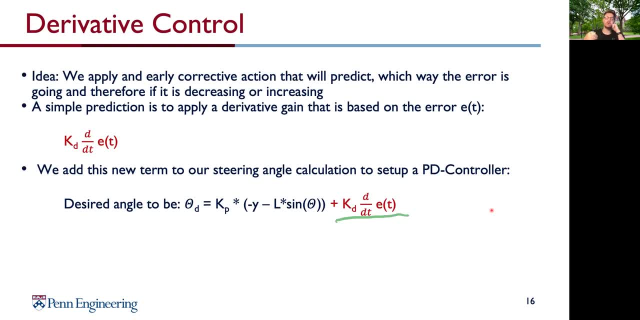 that creates a steering drift, it will cause a new and a big cross-track error and we will not achieve defining the centerline. in addition, the trajectory correction takes longer because it needs time to smooth out, which means, like in a proportional controller, we might just head our steering drive straight to the center. 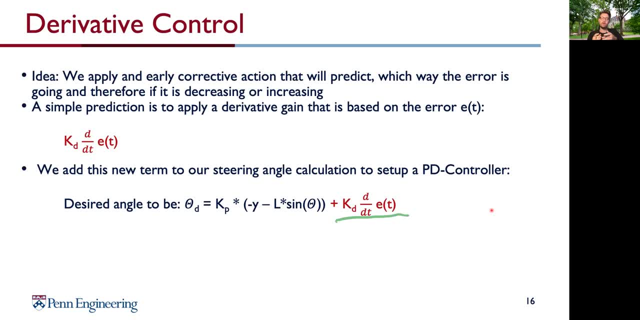 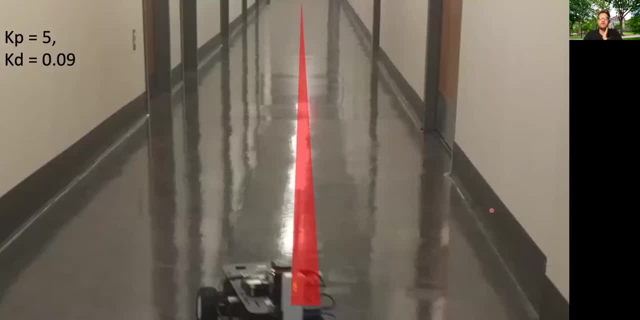 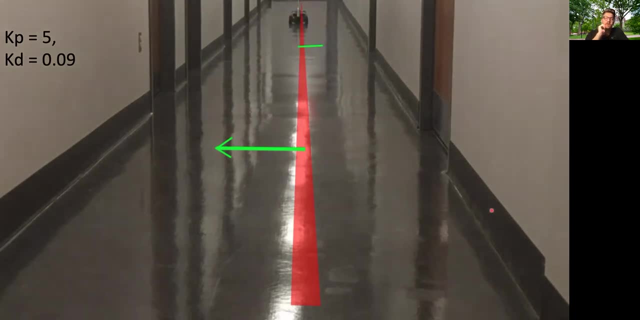 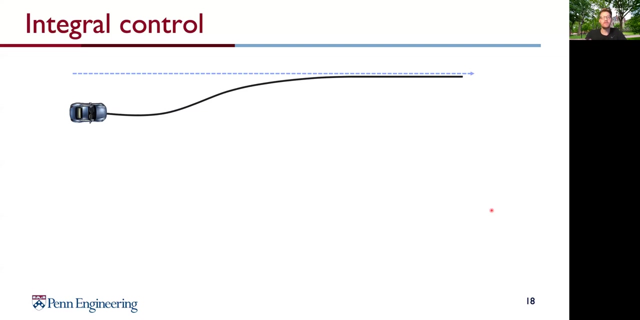 line but overshoot afterwards. now it takes a little bit longer and we are approaching the curve more slowly. so you can see here now a video where we integrated K, P and KT controller and the overshoot here a little bit too, but we are approaching our curve after our reference line afterwards. so P D 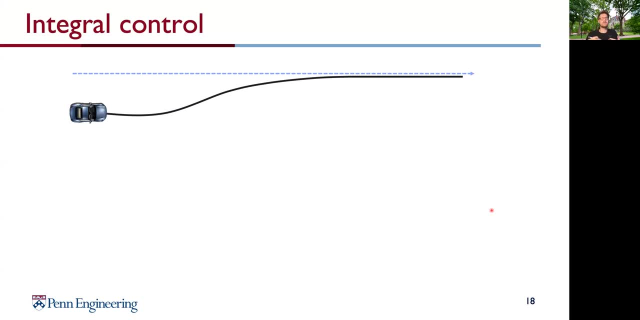 controller is now finished. now we're coming to the last part, because we are not really satisfied with with this set up, so we want to enhance it a little bit more. so again, we are driving here with our car, and imagine if you drive a car and your normal steering. 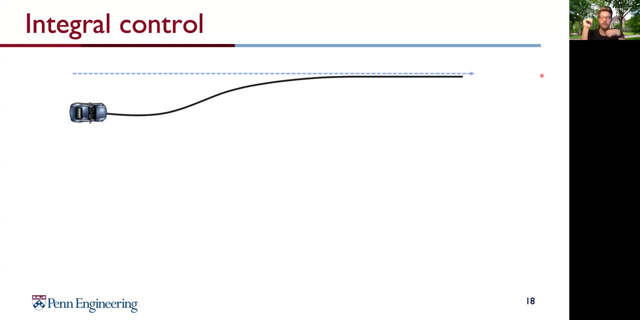 mode leads you to track theory, to a trajectory away from the goal. so then you normally realize for a specific period of time that you can't get closer and you would see more and adjust to the bias. and what do you need? what do you need for that? so you need a sustained situation of a large arrow and that 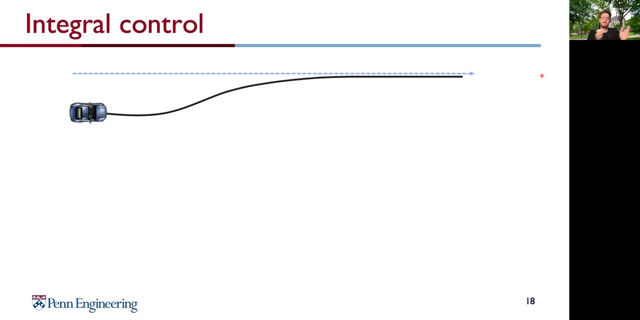 means we measuring the sum of our errors and that is not for anybody. so built in a the cross-tracked error over the time. so the idea is the steady state error accumulates over time and we apply additional correcting if you put that is sensitive to the total error. so far. so you see here now the additional. 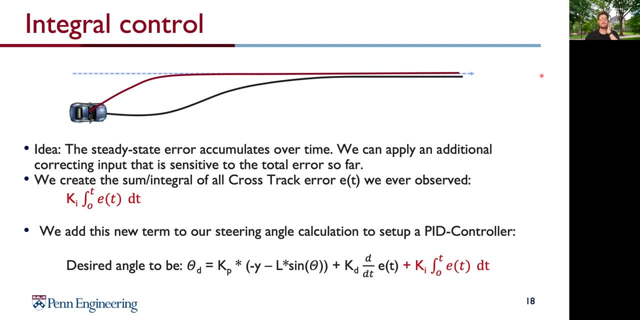 trajectory, our cards approaching it's much faster, it's going much faster to the reference line is sticking more closely to the reference line. so we add now the sum, or let's say the integral, of all cross-track errors et have an additional parameter, ki, which defines our gain and creating the integral over. 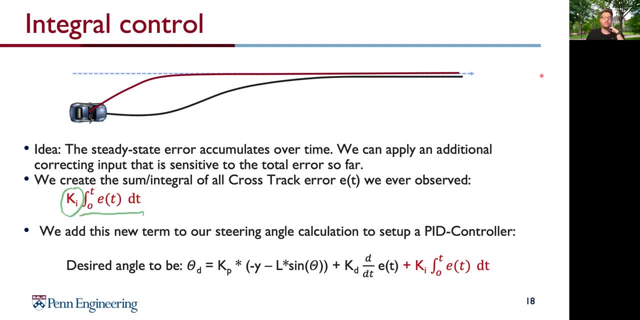 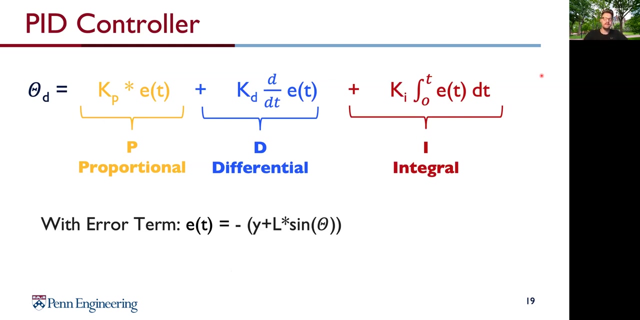 et and we add this term again. we created this one and edit now to our reference line, mathematical calculation, and with that we have all the parameters together to calculate a correct steering angle- theta- and with this setup we are good to go to drive more advanced. so to sum it up, this is our PID controller, based on the. 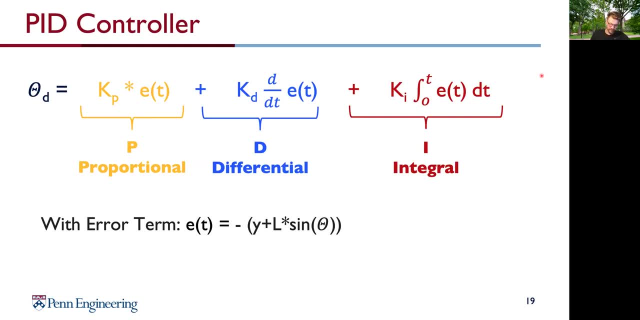 arrow E from T, and this arrow term is defined again by the distance to the reference line and the path along the wall, just in this case. so your term might be different, but this equation over here where you calculate the steering angle, you can apply that to all of the control problems you know. 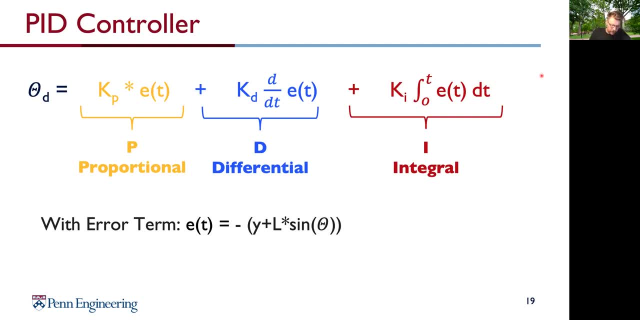 okay, and again, this is defined by the proportional term, by the differential term and by the integral chart. a PID controller- another term is three term- controller is now a control loop mechanism to employ feedback that is widely used in industrial control systems and a variety of other applications. and again, the PID controller. 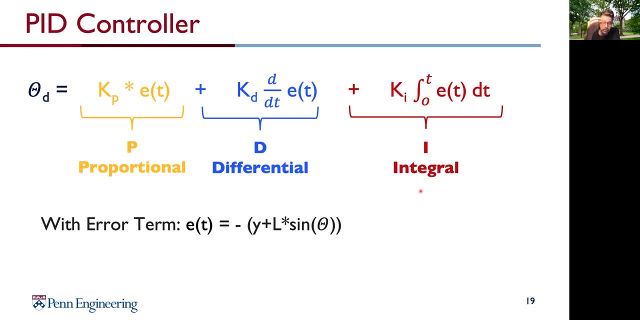 continuously calculates an error value E from key as the difference between our desired reference or set-point and measured process information, and he applies a correction based on the proportional first part, differential second part and integral part, hence the name PID. and here again I'm br broken PID. 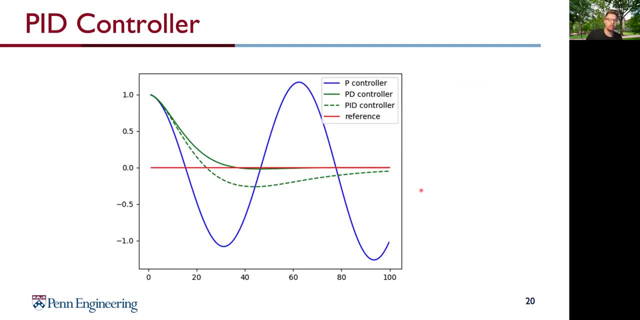 because we are planning the slope for the process if it were to work and as you can see here, you on simulation, where you see again that in red here is our reference line. we want to achieve that and if we apply different controllers we achieve different outcome of our system afterwards. and to see it on the car. 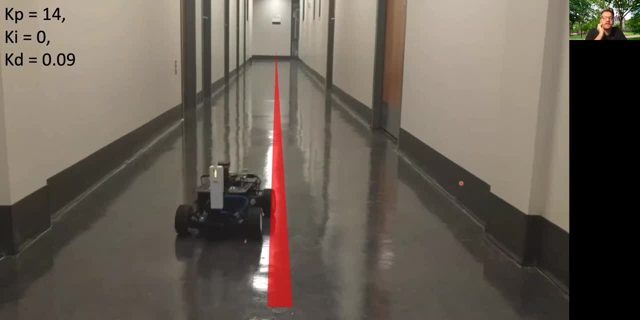 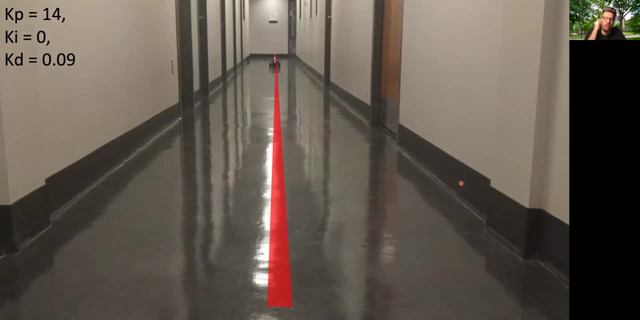 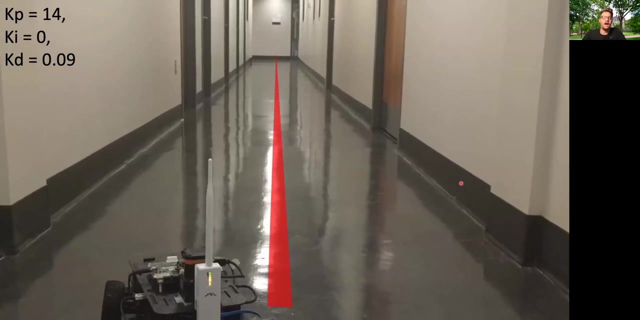 because you want to apply it on the car. here the car starts of the center with the direction to the left. the car starts and corrects very fast with like one overcorrection, and the overcorrection decreased in comparison to our first video. I will play that for you again just to give you an impression. but what? 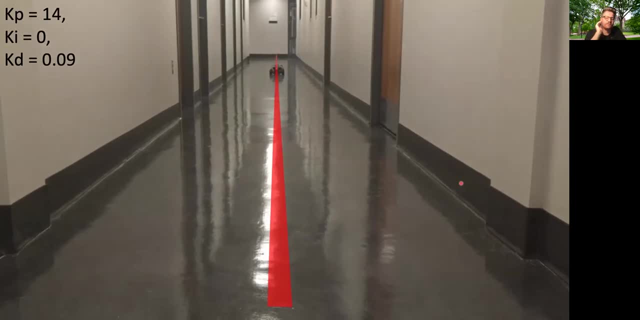 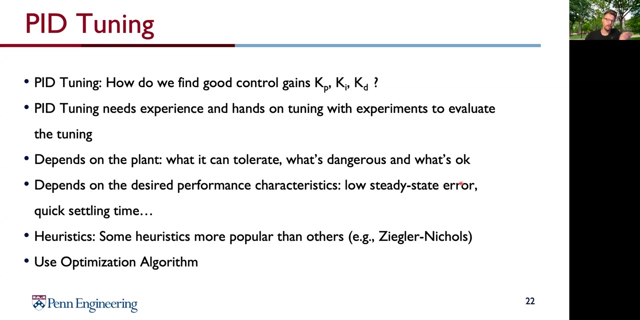 you just saw in simulation and now you can see it here on the real car. so now we learned how we can set up a PID controller. but what's the magic behind PID? it's basically the tuning, which means we can set up a PID controller. and we can set up a PID controller and we can set up a PID controller. but what's the magic behind PID? it's basically the tuning, which means we 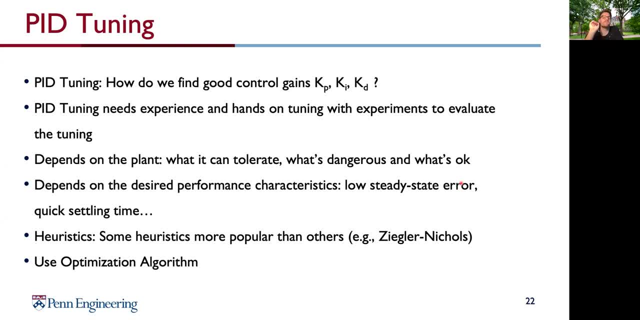 have to find good control gains. you remember each of the different parts. PID can an additional control gain, which means these are the parameters we can tune and these parameter can vary from system to system. so the tuning of PID controller needs experience and hands-on tuning with experiments with 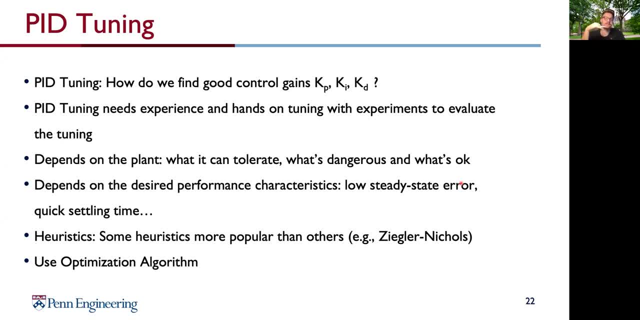 simulations and, in addition, it depends on the system you have contains these parameters and importance for your system so that, in addition to this, we can set it up. and let's look at the PID controller which is designed to do things like this, a PID controller for our electrical engine, which I showed you. 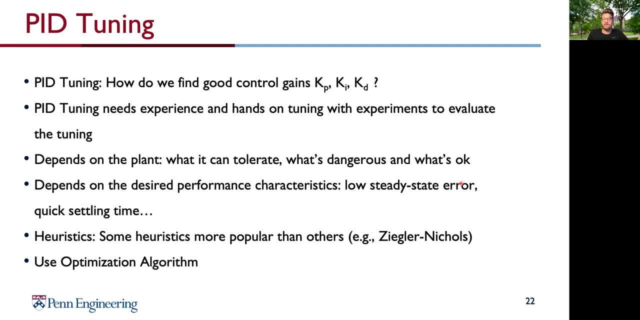 in the beginning might be different from the PID controller of our reference tracking. in addition, what can the system tolerate and what's dangerous and what's okay for our system so it doesn't create or doesn't lead to a crash and in, And what we can use are two things. 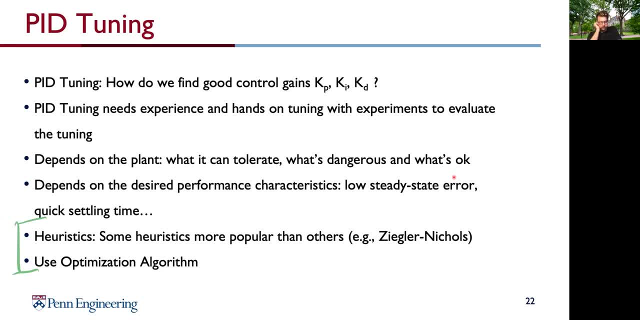 we can recommend you here. First of all, heuristics. There are heuristics we can use, for example, the Sigler-Nichols method. We put additional material there. You can read about that. Or you might just set up an optimization algorithm. 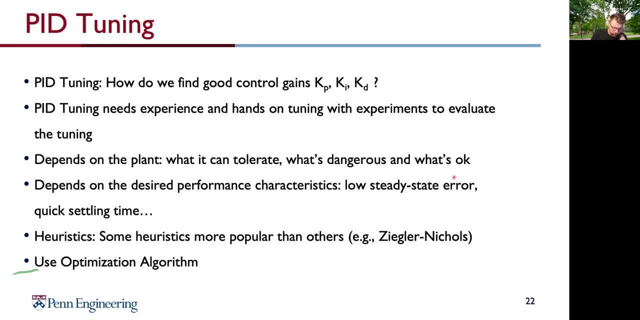 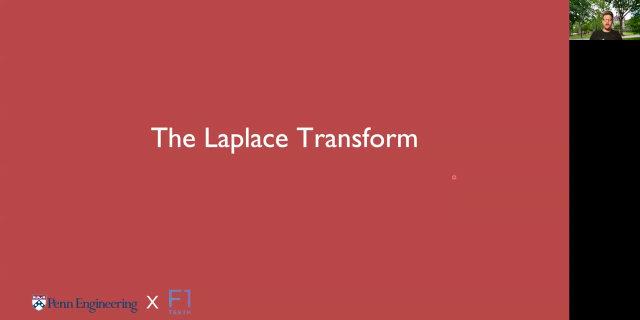 For the PID controller of your F110 car, it's probably enough to use the heuristics, like the Sigler-Nichols method, But for bigger systems we might use an optimization algorithm. So to sum it up, you just learned what a PID controller consists of. 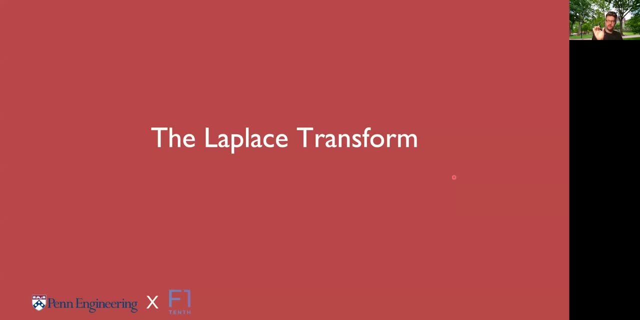 and that the main parts is the error and the control, gain parameters and the combination of both of them in a derivative, integral and proportional part leads to a PID controller. So Let's move the comment to our third part, the Laplace transform. 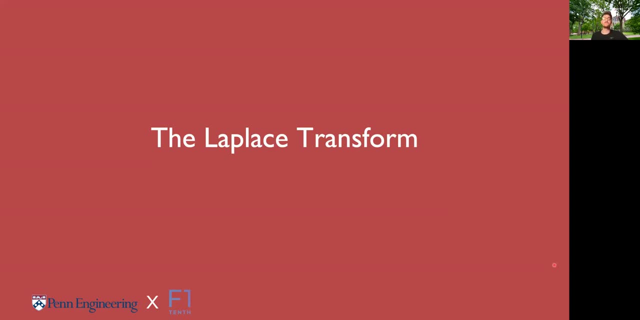 So I said to you at the end that we have to tune our system, that we have to do experiments and that we have to get like an insight of our system. Of course we can just apply to our car and drive with car and see afterwards what it's doing. 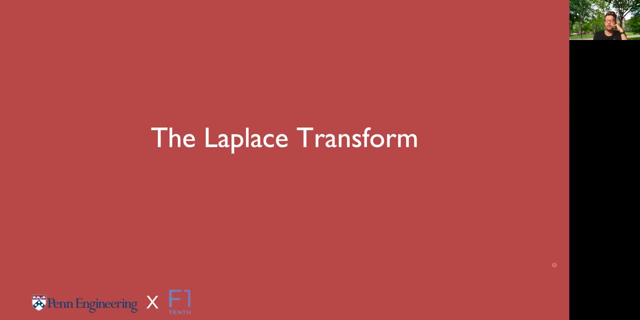 But this is like taking us a lot of time and we need the hardware. but we can do it. We can do it like with mass only and in simulations a priori, And to do that we are using something called the Laplace transform. 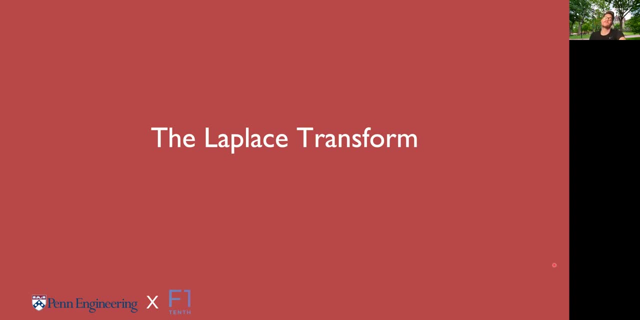 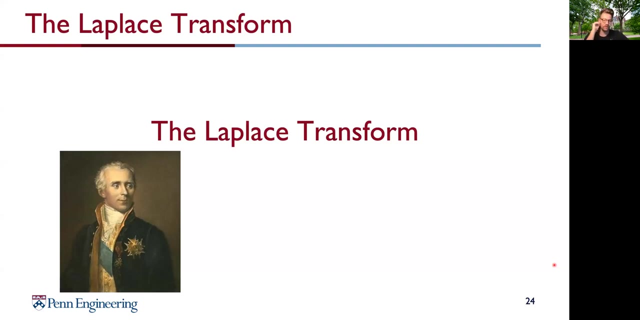 Perhaps you remember this also from control engineering or from your math courses, but we will wrap it up here. So in mathematics, the Laplace transform is named after its inventor, Pierre-Simon Marquis de Laplace, And What he's doing or what he invented? 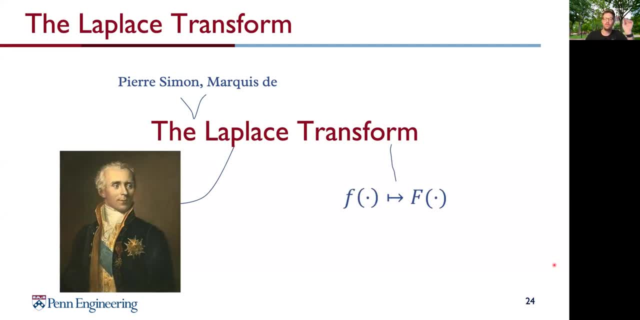 is an integral transform that converts one function of a real variable- t, or often called like time. t is time- to a function of a complex variable or a complex frequency. So this is just the basics. Like we transform one from the time space. 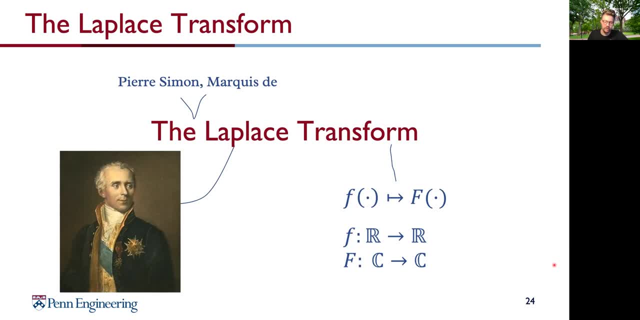 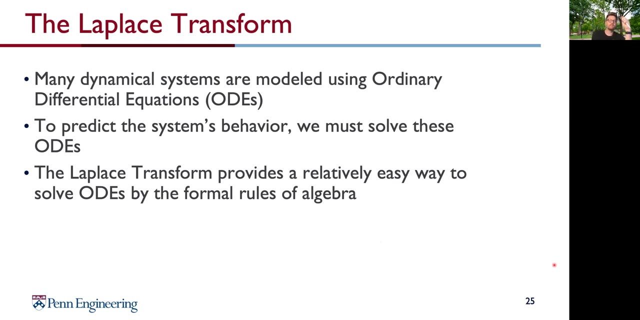 to the complex space, or what we call the frequency dot Time domain, frequency domain. This is what we achieve with this math And, first of all, why we want to do that. So many dynamical systems are modeled or displayed by ordinary differential equations. 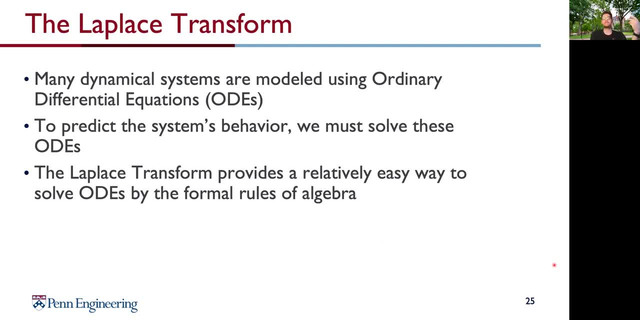 so-called ODEs To predict the system's behavior. we want to solve these ODEs, And the Laplace transform provides a relatively easy way to solve ODEs by the formal rules of algebra, which means we're transferring something. 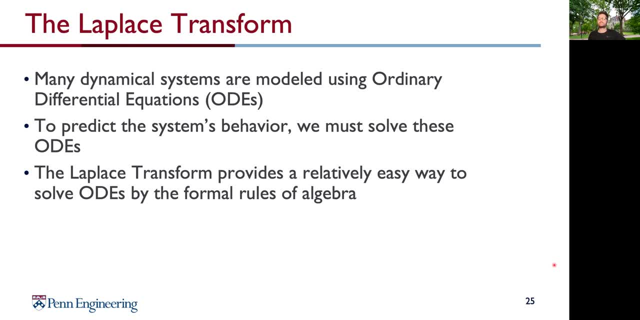 from derivative terms to simple polynomials, which we can calculate very easy, And in practice, however, one has to deal with systems that one doesn't know in principle and whose properties should be measured first. This is also really big issue here, So to give you an example, 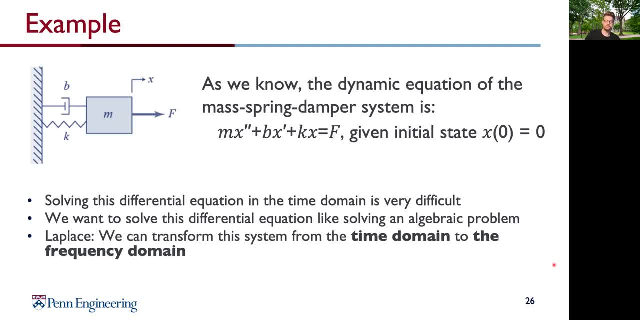 this is the well-known mass spring damper system And we can see here: we have a mass in our system, We have our damper coefficients, We have the spring coefficient And the movement in X direction of our math is applied by a fourth. 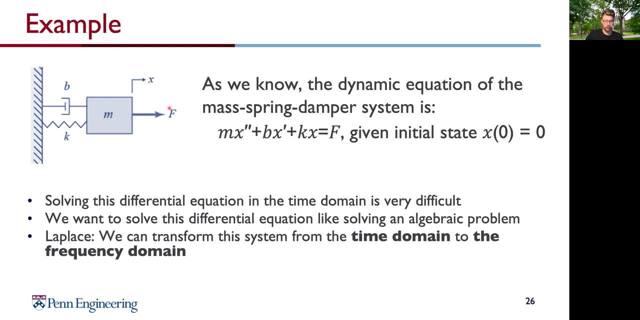 We can set up an equation, a differential equation, for that, which means we calculate. we calculate, multiply the mass by the second derivative of X, acceleration, and there the multiplication of the damper spring by the velocity, second derivative of X, as first derivative of X, and we multiply K with the X factor and this equals the. 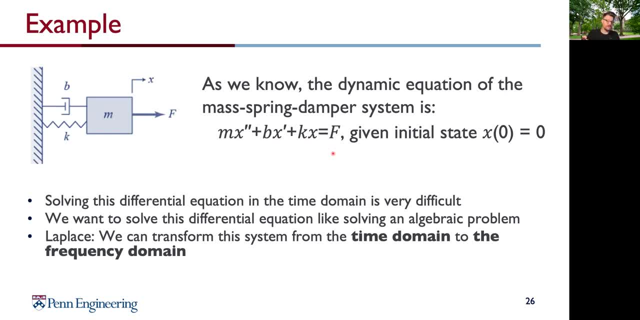 first. so we can set up this differential equations. but to solve this in our time domain is super difficult. so we want to solve this differential equation like an algebraic problem. again, here we transferring it from the time domain to the frequency domain and then we have a polynomial we can easily solve. so we 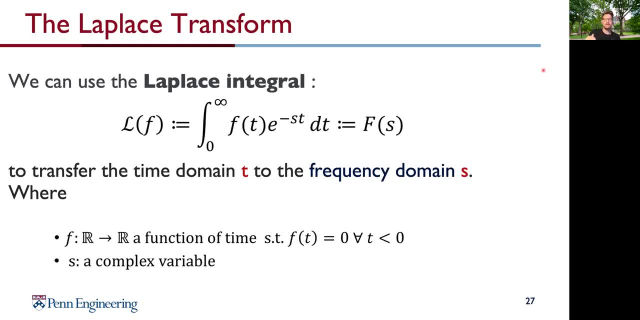 have a look at the mass. here we are using the so-called Laplace integral. for the Laplace integral you have always this variable here that looks like an L, which means we applying the Laplace integral to our function F and which means we multiply it by e to 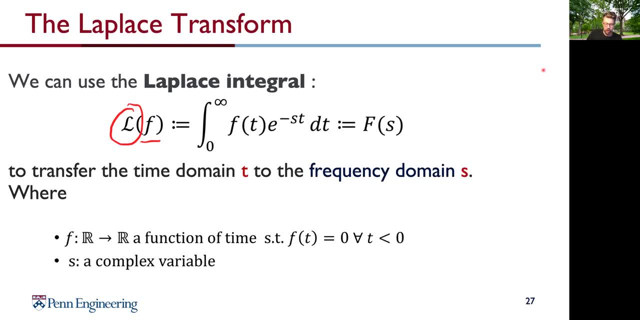 the power of st, bring the integral over the complete function and create therefore our transfer function F from s, as which is essentially the die, and E plus S plus t, and this is obviously the, the relative time that I just seen here, which is right. here you see the. 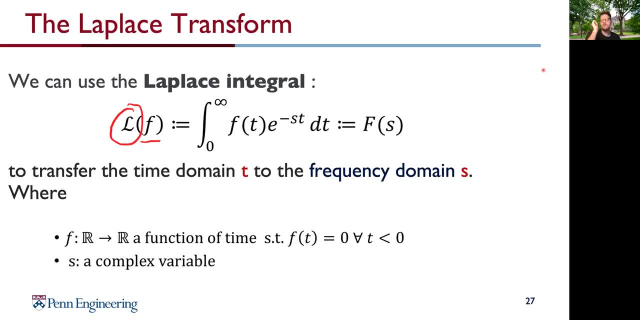 ppeutics with its perfect slice of las pages, what I need to do to simplify the躍 of the lactate. I wasn't the Datenbold from yesterday. I need to remember the ر and τ Kam количе are plotted over the time t and for the most common differential equations to 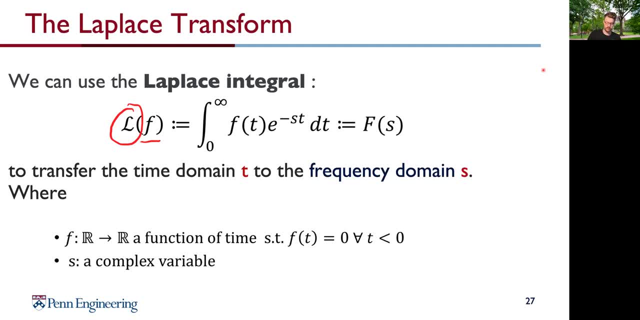 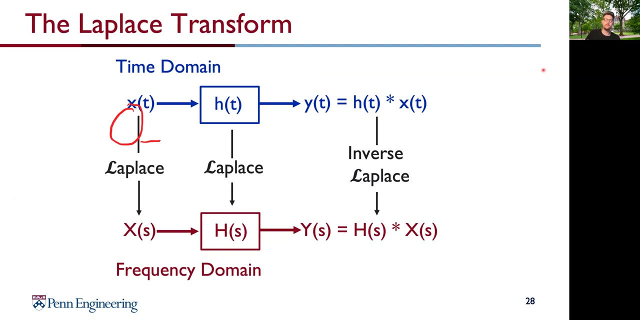 calculate the reversible unique image function fs. So to repeat it here again, we have something that is existing in time, domain t, and we transfer it with the Laplace integral to the frequency domain. And here is an overview again of that. we have an input x, we have a plant and a function and we 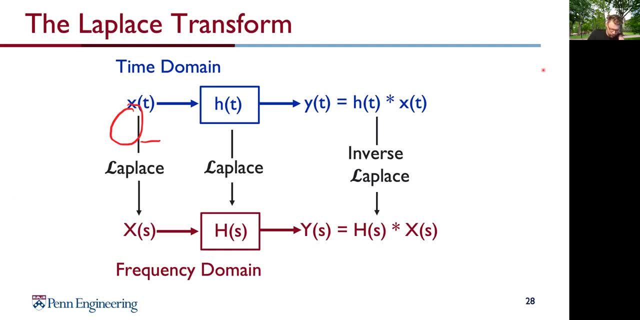 have an output y And with Laplace we can go here over the system, which means x is transferred to x from t, transferred to x from s, Our plant h from t is transferred to h from s and our output y from t is transferred to y from s. 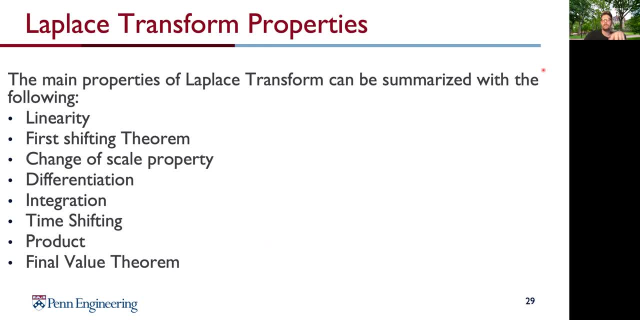 the mass behind the Laplace transform or the transform properties. we won't, we will not show you today because this is like basic mass or basic control engineering math and we will just fresh up your knowledge here. so the Laplace transform will relies on main properties like the property of 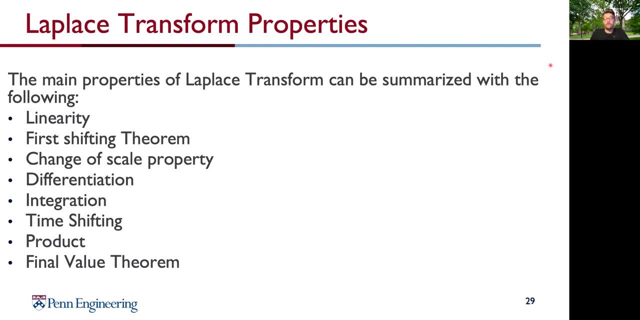 linearity, the first shifting theory, the differential integration, which means there are specific properties, how you can transform your normal math or your normal differential equations to the Laplace domain. now, for example, we will have a look at the linearity part, just to give you an example here. so 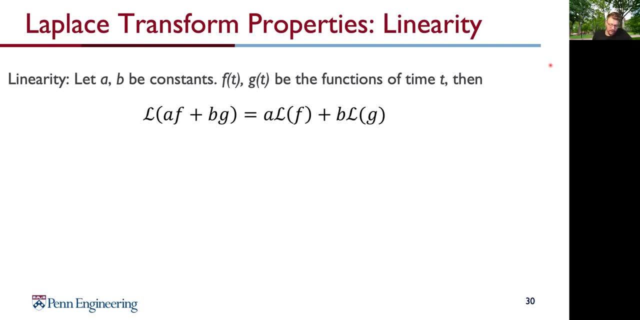 we are now having a function, F from T and G from T. both of them are in the time domain. we have a and B that are constants in our systems and we want now make a Laplace transformation of the complete function and what we say that we can put out or like push. 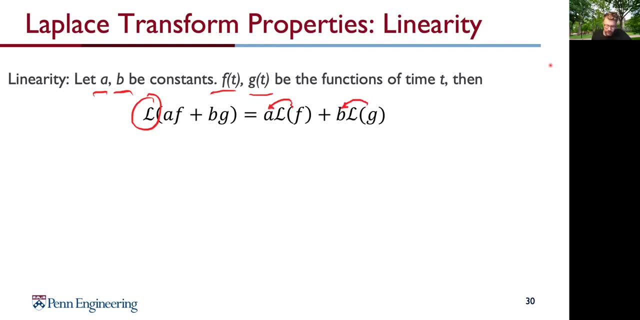 out both of the constants here and say it's the same if you just pull them out and make the Laplace transformation on the functions itself. so now you can just believe me with that or what you can also do. you can prove it. we wrote down the proof for you. where we did the Laplace transformation for you- here you can have a look at earlier task�was here, and now what we are finishing the Laplace transformation for you. here you can have a look at those two. okay, we then take a small stretch here. you can see, in order to finish this, there is only two夠 to complete it. so we will tell you now a little bit of a tutorial, but all in all, for now, 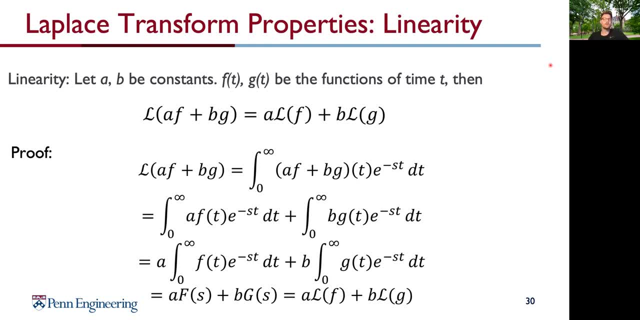 you can have a look at this more detail, but more or less, we are proving in this case again that this is the same so which means there are specific properties. so before you start with transferring something into the frequency domain with the last Laplace transformation, please make sure that you. 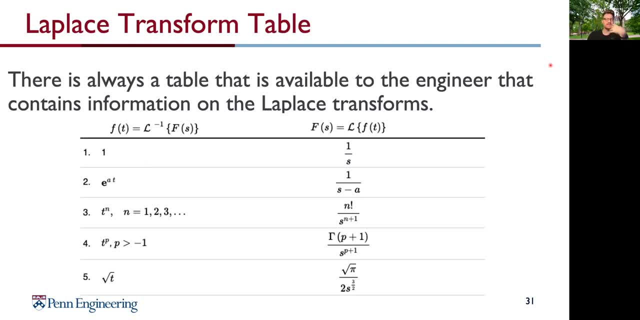 know about the properties. in addition, for us engineers, there is always a table that is available which contains information about the Laplace transform, which means if we have a specific value in the time domain, for example one here, our constant one in the time domain, this is displayed. 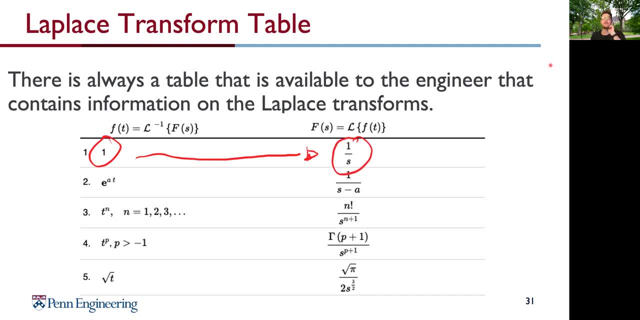 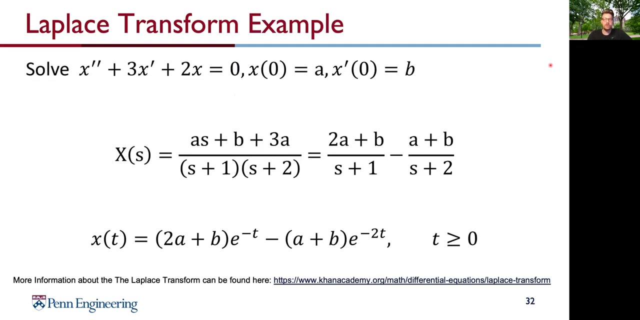 as one divided by two, by our complex number, as in the Laplace domain, and for all mathematic expressions. we have here different transfers and you can have a look at this table. to make your life a little bit easier and just for the completeness, we brought here one example to you. I will not go here into detail. 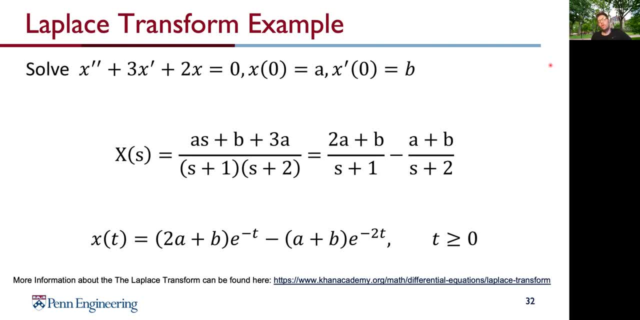 but we showed you here that we have one differential equation and we set up the Laplace calculation for you here which you can solve. but an additional link gives you more information about the blood class transformation here. we will not go here in detail because, like this is just a refresh of you to show you. 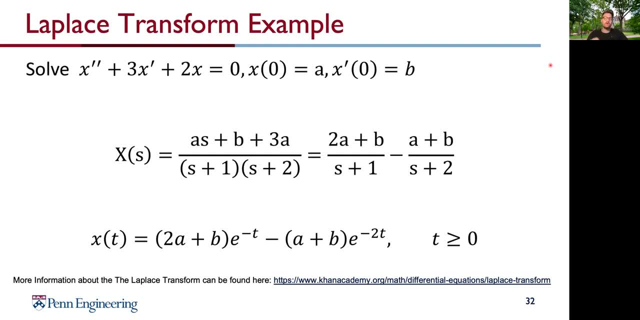 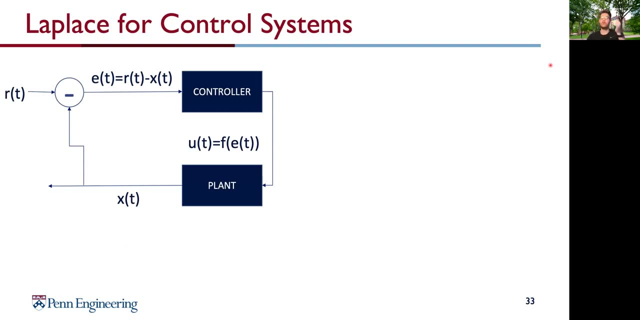 what is possible, because we want to use this example to show you what is possible. because we want to use this example to information, to set up our Laplace domain or our frequency domain for our control system. so what we do is we have now our control system here. remember we have the 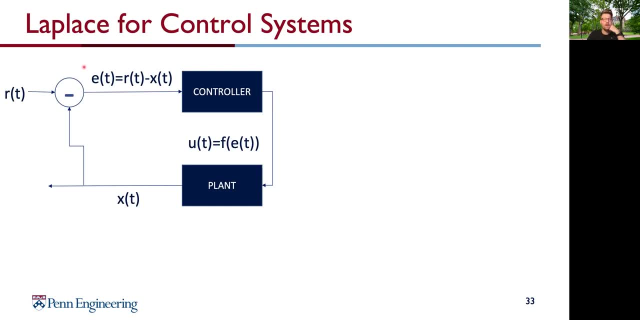 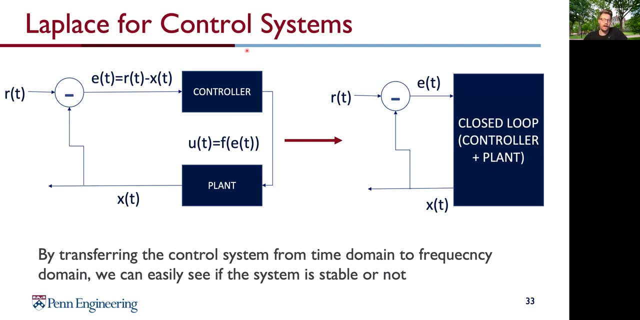 reference input. here we have our error. we have our output signal, we have to control input signal and we have to control and the plan. so first of all we setting up our control system, we have to control and the plan. so first of all we a closed-loop system, so we have the controller and the plant in one. so it's 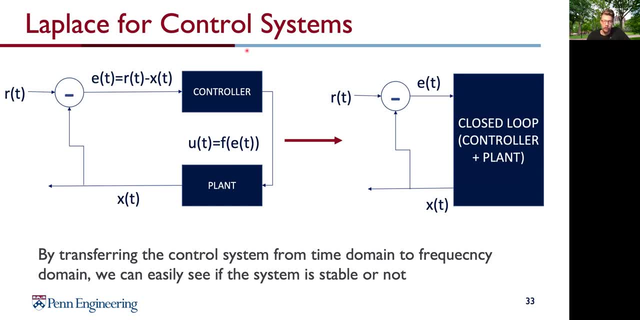 a little bit more compact. and what we do now, we are transferring. sorry, we are transferring or we are creating a transfer function. the key advantage of the transfer function is again their compactness, which makes them suitable for frequency domain analyzes and stability studies afterwards. so the transfer function itself: it suffers from neglecting. initial 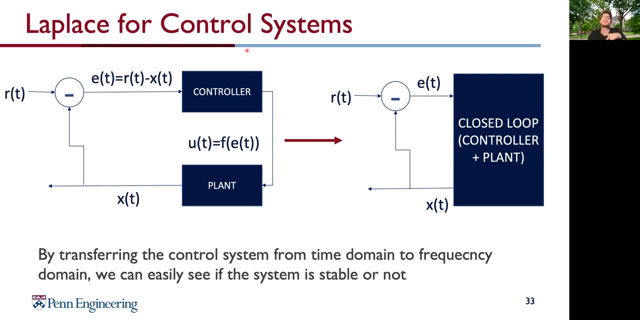 conditions. not only does the state based representation serve as an alternative to this transfer functions, but although it is not limited to linear and time-interval system. and it has fallen vents. and then again, by transferring the control system to the from time domain, to the frequency domain, we can easily see if the system is stable or not. but 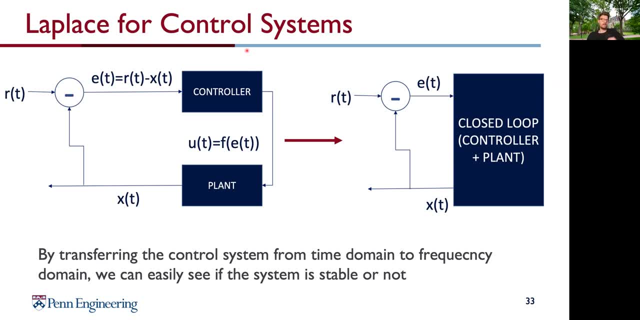 remember here. I will say it at the end again: stable in this case means that our control- sorry, our control output is controlled, so it's not like getting bigger and bigger and bigger and leading to an uncontrolled system again. so we are creating here the transfer functions and our control loop. 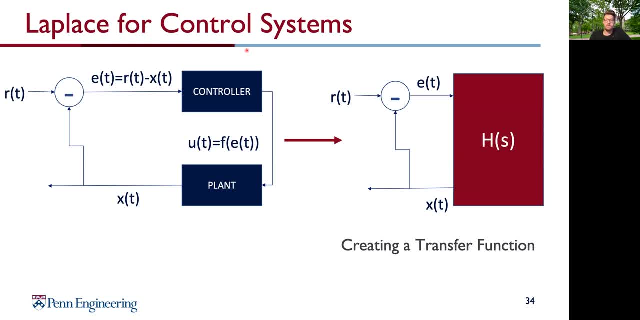 consists here of our- yeah, several interconnected blocks again, and by transferring it to the frequency domain we can describe the whole system with one transfer function only. we have here displayed you in red and for the interconnection of the rules, sorry for the interconnection of the individual blocks. we will use the rules, what we saw. 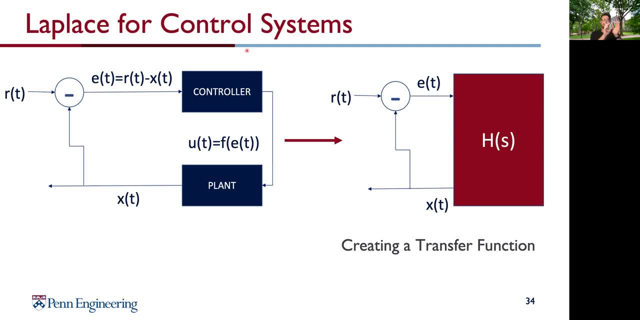 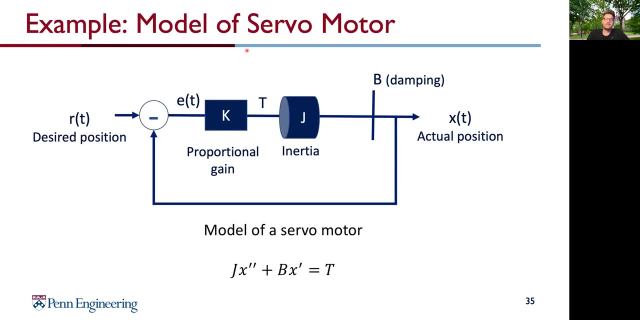 before. like, we have one number, one variable in our time domain. we use the transfer table we transferred, we make the calculation, we make the math and create our transfer function afterwards. so, for example, this is the model of our server. here you can see the complete model of the system, which is modeled in the time domain, and it includes both plant and controller. 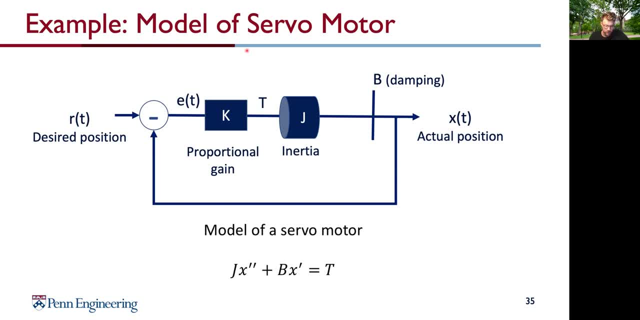 because we have the controller part with our proportional gain. here we have the error and we have the modeling, the plan modeling of our motor, and we can set up here again our differential equations. but, as I said before, we want to now transfer this one from time domain to the frequency. 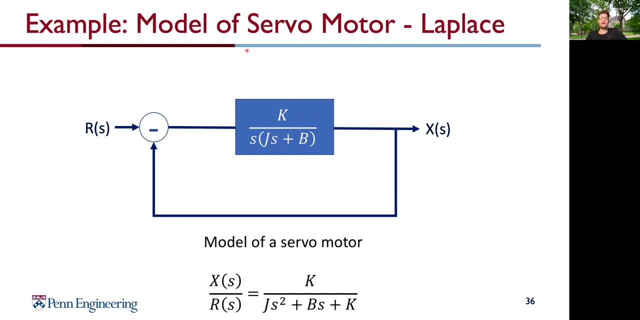 domain. and here we see now the example of the motor system transferred to the frequency domain. that includes both motor model and the controller, and what we can see here, the what we always have, the expression is the output divided by the reference and where we display here our transfer. 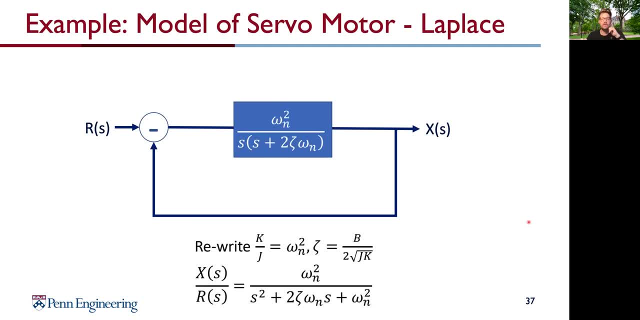 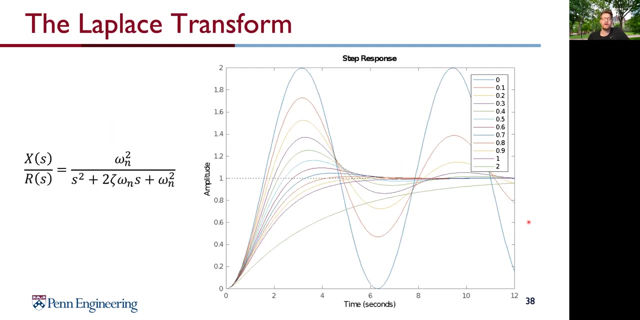 function only what you can do afterwards. we integrate the real value variables for it, like here the rotating end and speed, so we can rewrite our- yeah, let's say, variables only with real physical parameters to express a calculation afterwards and to have a look at simulations. so you, what you can see here. 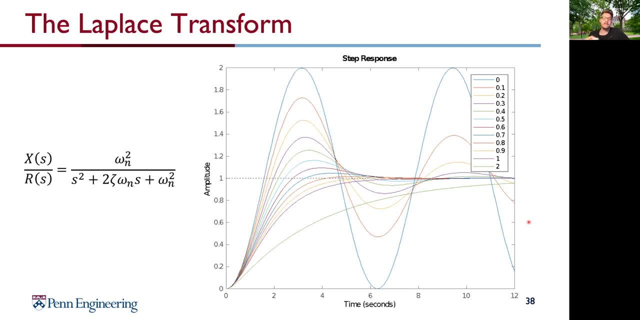 is that we see the step response of our system. so what we have done, we applied an input to our calculations and we see a step response of our engine afterwards and what we can see. if we apply different parameters we get and different output of our system afterwards. so the acquisition of the properties, that can be done by recording step and 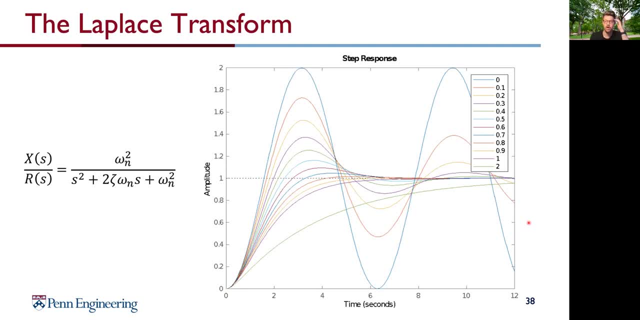 pulse responses. what we can see here is the step response or by measuring the frequency response: step response, impulse, impulse response, frequency response. and the original differential equations have similar informations for us because they all contain this description of the system in different form, and remember that again why we are doing that in our differential equations. 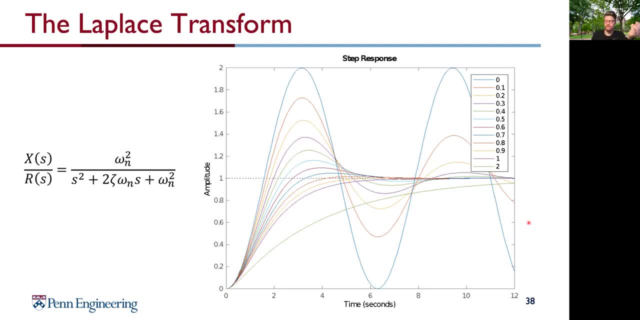 it's difficult for us to solve the system here in the Laplace domain. we have this simple calculation on the left side where we can apply the real parameters and we get an output afterwards and this we can plot and then analyze and the saying what we can do for our 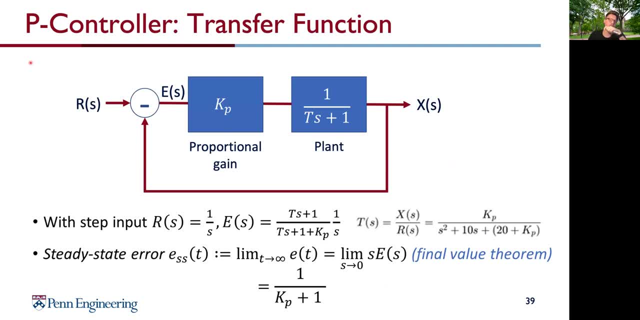 models itself is then for our controllers, like, displayed here, the P controller. it reduces the rise time, it increases the overshoot and it reduces the steady-state error. the proportional controller in the Laplace domain is no more or less the error multiplied with a factor KP. what 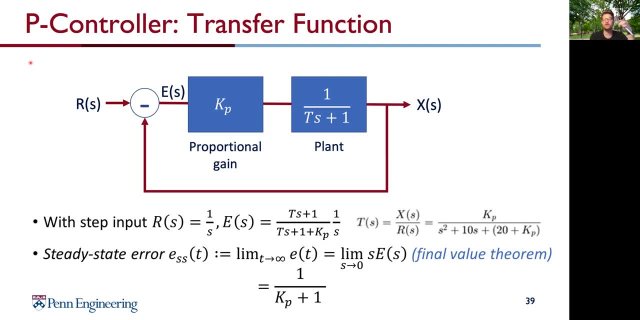 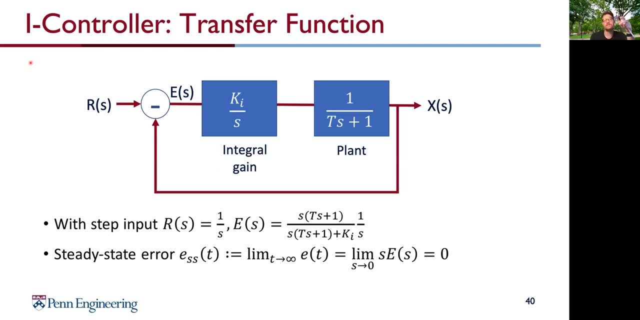 you can see here the closed loop transfer function of the above system with the proportional controller is then TS. what you can see down below, and you can do the same with your integral controller, and we can see here again: if you're applying one specific input, like here you, we are applying. 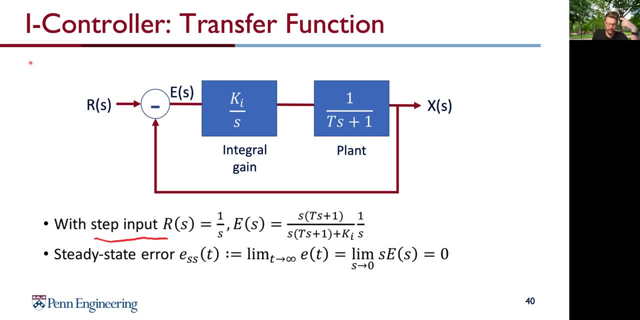 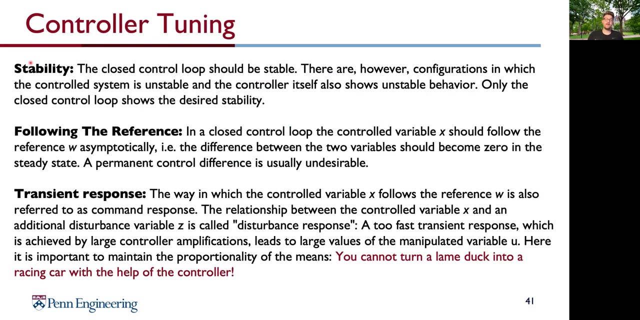 a step input to our system, which is defined in the Laplace space, again what we saw before as one specific parameter in time domain and in a frequency domain, one divided by a single parameter, by s, and we create an arrow for that again and can create a transfer function afterwards. so again, why? 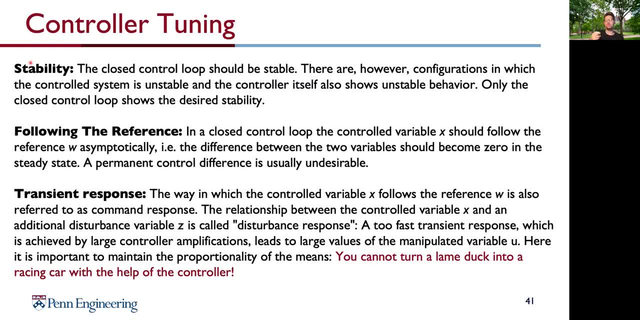 we are doing this because we want to tune our controller, we want to figure out the individual parameters for our control game, KP, ki and KD, and we can analyze our system. regarding the stability, again, the system is said to be stable if its output is under control. otherwise it's said to. 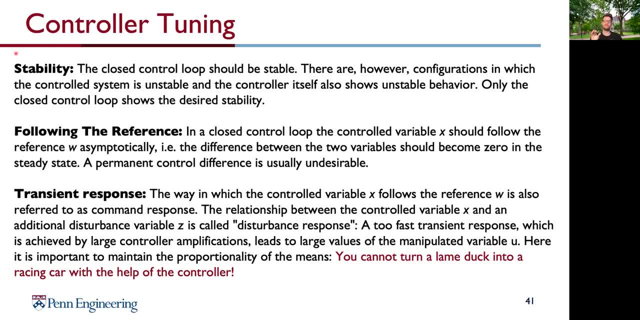 be unstable. a stable system produces a bounded output for a given bounded input. so again, it's not just like that. our output is getting bigger and bigger. in addition, we want our system to following the reference quite fast and easy and smoothly and we want to have a transient response here and with the creation of our laplace transformation. 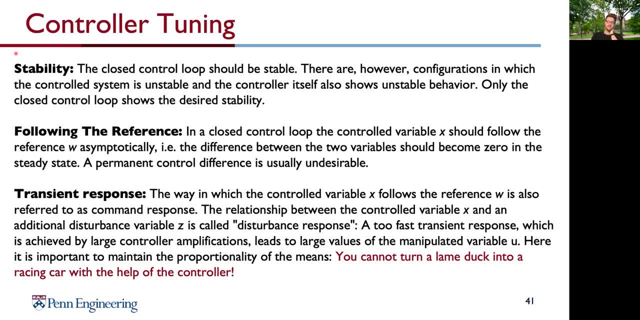 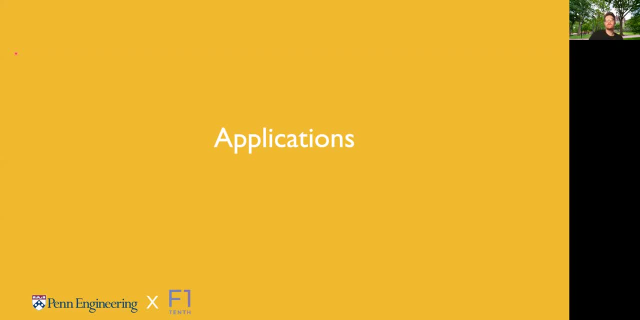 from the time domain to the frequency domain. we create the possibility that we can analyze a function and tune our system afterwards. so this was a lot of input. this was a lot of math input for you and I think if you, if you have now to remember all this stuff again from your, 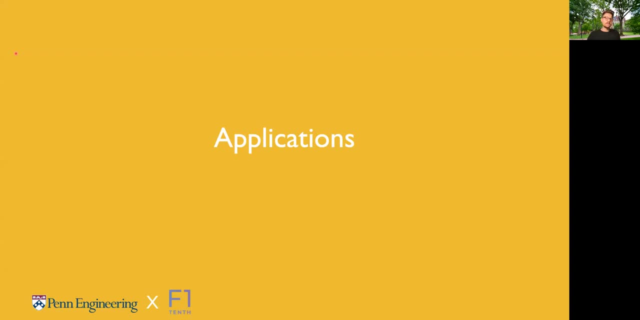 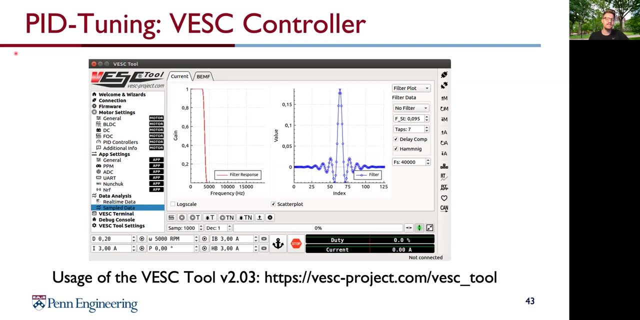 control engineering lectures. so we will now wrap up everything we learned in the past 50 minutes and apply it to one specific function, and we do it with a little help so you can do it more easily and faster. we are tuning now our motor controller, our motor. 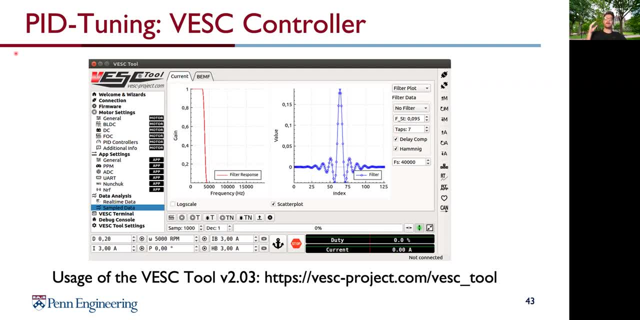 controller is consisting consisting of a P and I and D part, which means we have a P ID controller here and we will use a tool for that, the so-called VSC2. you can download it here. and this B еще gives us the policy ability to connect our control system to the trolls web and railroad traffic rules. we can see how fast or how fast that is, so let's connect our vsc source on pid device. so we'll do our little: teleport and password comma and set-up our and no document in 20 and a whileо. 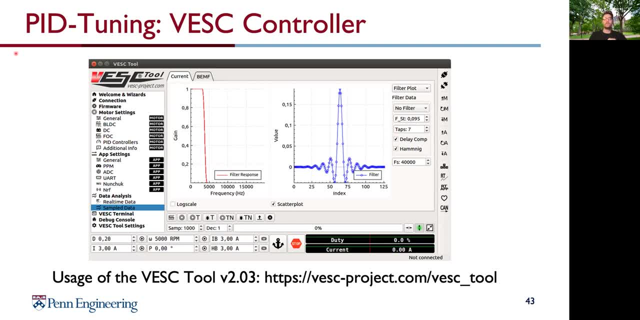 to connect our computer with the motor controller of the electrical engine of our f1 10th car and after you did a firmware update, you can select our motor configuration we created from you. it's in an XML file. what you can do. you can just drop it in here in the VC system and you write it to. 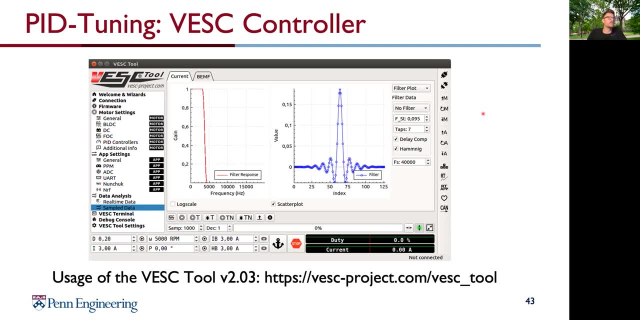 the motor configuration and what you can see here is the down arrow and the M and with this one here you will download your current configuration to the engine. if you create new variables, you create a new motor configuration. we have to download it again. so note: in the future you'll have to press. 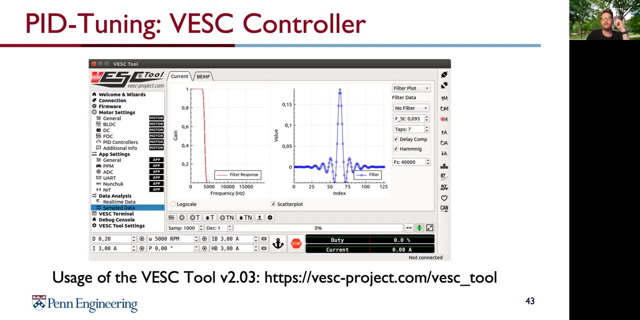 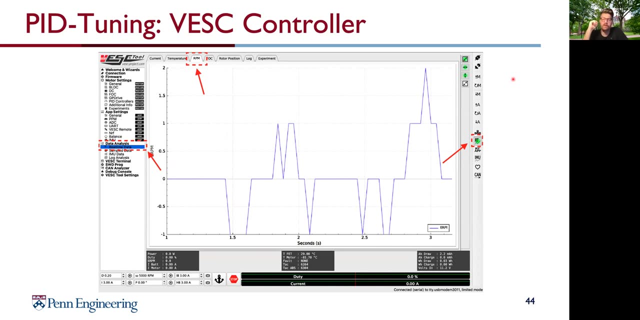 this button whenever you make a change in the motor configuration. without that, it's not getting applied. so, but this is just a set up and you will find more additional information in the tutorials. so what we do? we start tuning the speed pet controller. this PID controller controls the speed of our 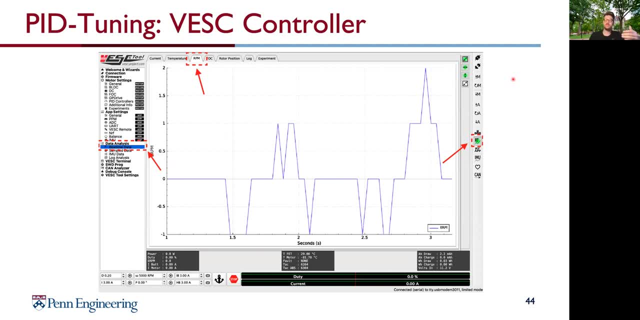 engine, which means I give the information that I want to have 1000 rpm. the controller of our motor controller achieve this for us and we can do this in our engine. this but this is not otherwise. we have to create Bear demos that are can tune that so to see the RPM response from the motor navigate to the real-time. 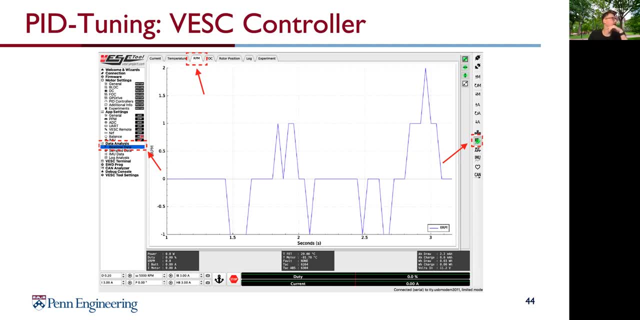 data tab under data analyzes on the left, what you can see. here you have different information about the system, like the current the motor is draining, the temperature of the motor or the RPM or the rotor position. so all useful information. and to click the stream real-time data, you can click the button. 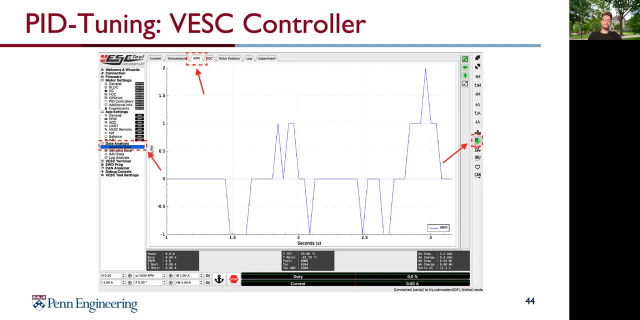 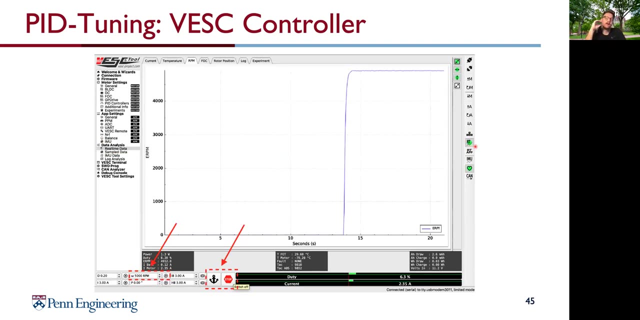 here on the right, and then you can actually put the car on table, activate your your motor with your wireless controller and see the real-time data of the engine. so again, we have now our system, we have now a controller and we say we are not happy with it. 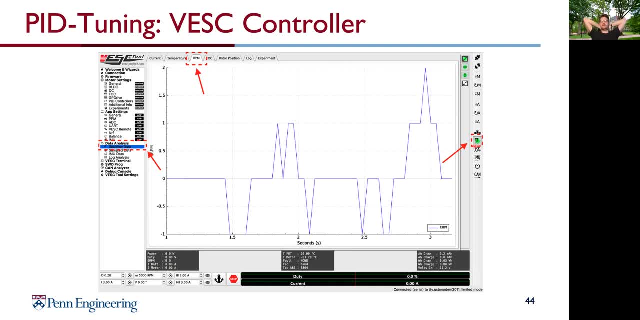 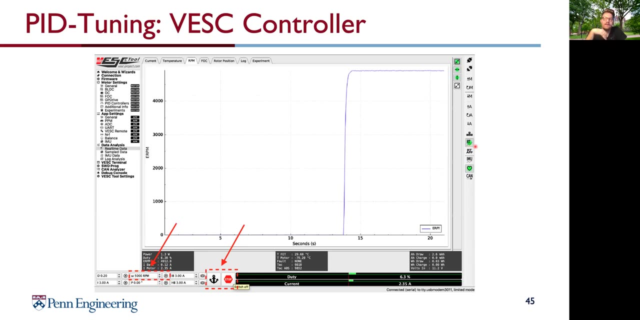 so what we do? we gain measurement insights to our system with the real-time data stream, here and now. it's time to tune it. and again, what are we doing? we are applying specific signals, for example, the so-called step response that gives us information about the system's behavior. so, to create a step response: 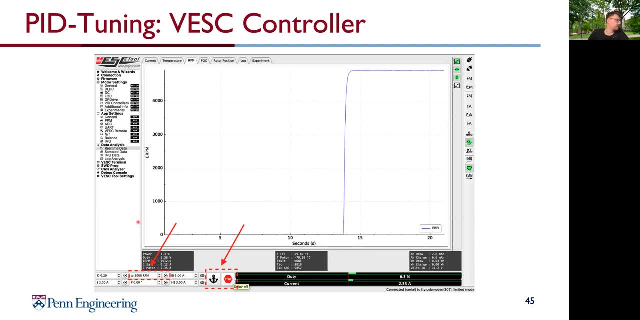 for the motor. here you can set a target RPM. we create that here. a target RPM is a step response for the motor. here you can set a target RPM. we create that here, a target RPM. you can choose between two thousand, ten thousand rpm. then you click to the. 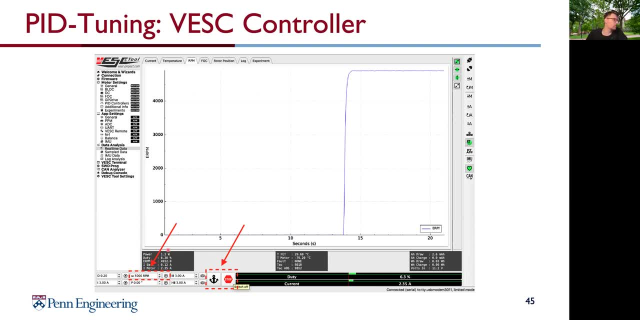 button next to the box to start the motor, which you can see here, and be careful about that because the motor will spin afterwards so you make sure that the wheels of your vehicle are clear from objects and is not located on the ground. the enter: click the enter or stop button right next to it to the 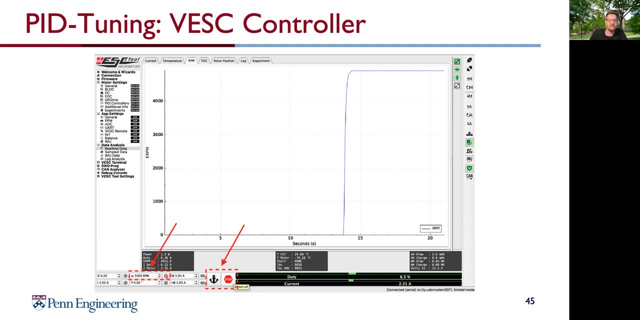 sorry, and this is for stopping the system. this for applying step response and you can see here now the measurement of the step response. so here's the measurement: our motor is not doing anything. we have the step response, which is really high and then goes up to five thousand and we can see the behavior of 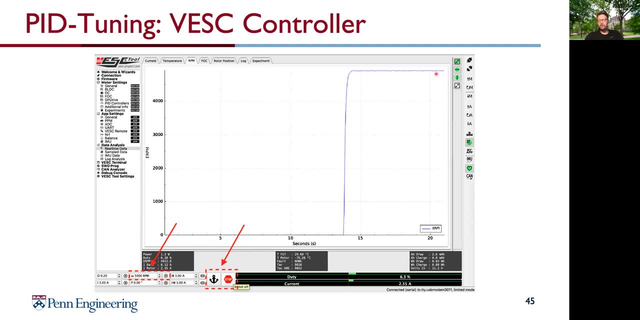 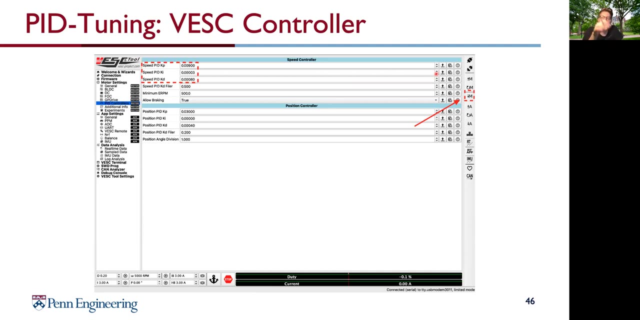 the engine afterwards. you want to look for a clean step response that has a quick rise time and zero to very little steady state error, and then you can inspect the system and you can adjust the accordingly by the navigating to the BIT controllers under the the motor, here PID controllers. you 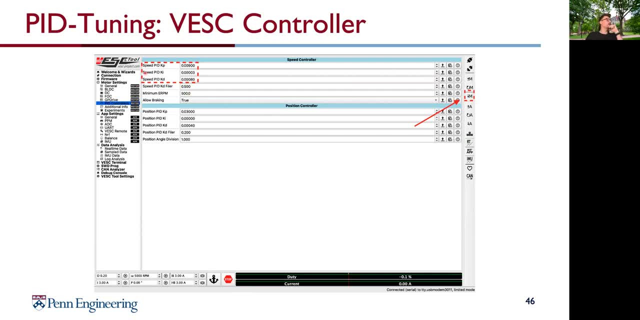 see here your KP, your ki and your KD parameters. you can change them and apply to the motor again and with the roots of tuning I told you before like, either it's an optimization or you just use the heuristic, you can gain them and apply them and if you're seeing a lot of